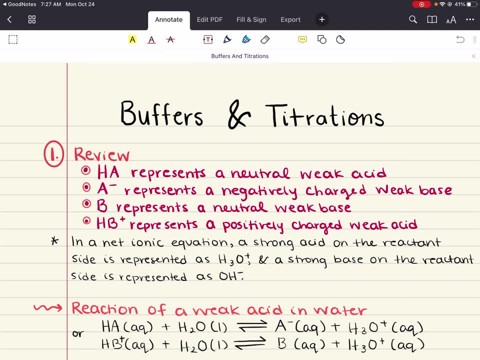 Hello everybody, my name is Iman. Welcome back to my YouTube channel. Today we're going to be covering chapter 15, which is all about buffer and titrations. Now, if you remember, equilibrium principles, help us understand many processes that take place in aqueous solution. One example that: 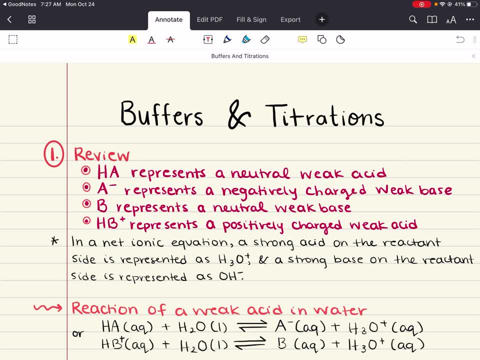 carries important implications for our health involves the pH of our blood. Our blood needs to be maintained at 7.4, and it is through a process known as buffering that it makes it possible to do that. We're going to be talking about these buffer and titrations in this chapter. 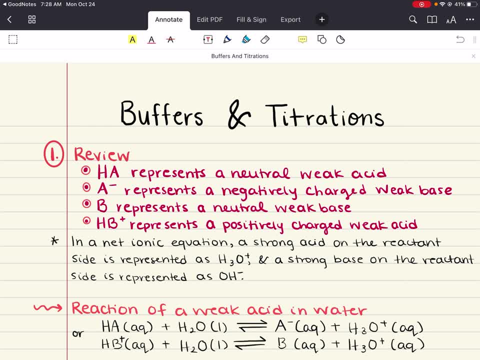 so hopefully you'll understand how that is possible. Now in this chapter we're going to extend our understanding of acid-base chemistry in aqueous systems by looking at buffers and acid-base titrations. We're going to also describe the equilibrium behavior of saturated solutions of sparingly soluble. 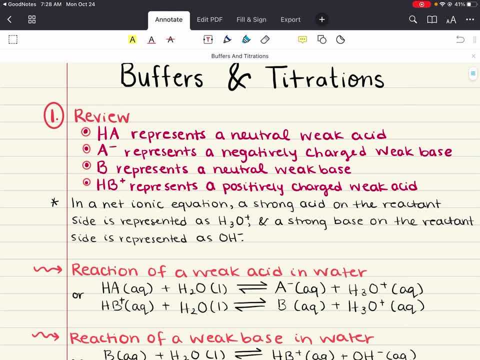 salts using another equilibrium constant, which we're going to call Ksp. Now, before we get started on all that new material, let us review what we've spent a couple of lectures discussing in order to solve acid-base problems and what we'll use to solve buffer and titrations problems. 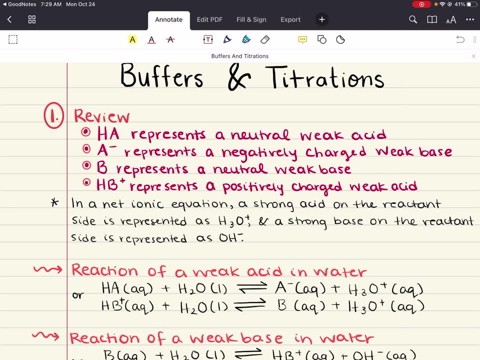 In order to do that, it's important for us to identify the appropriate chemical equation. For example, if you're asked to determine the pH of any aqueous solution, you should focus on the reactions occurring in the solution So you can say that the relevant acid-base reactions can be summarized. 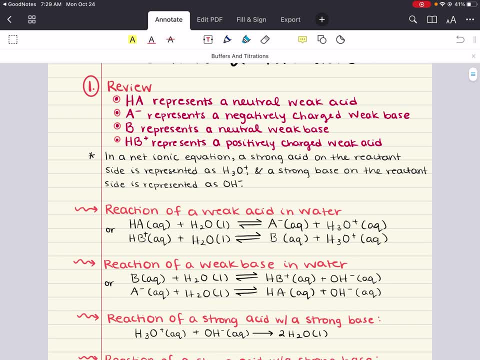 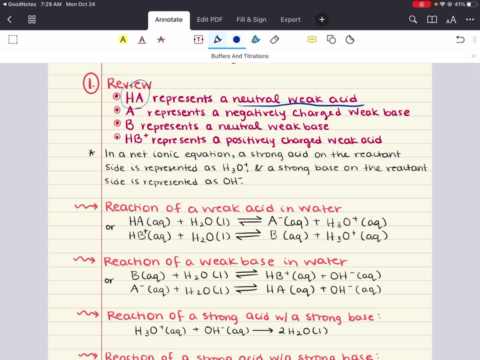 as well HA. When we see HA, usually what we've been writing for HA is that it represents a neutral weak acid. Alright A- here represents the negatively charged weak base or the conjugate base of our HA, of our acid. Alright B represents any neutral weak base. HB- represents our positively. 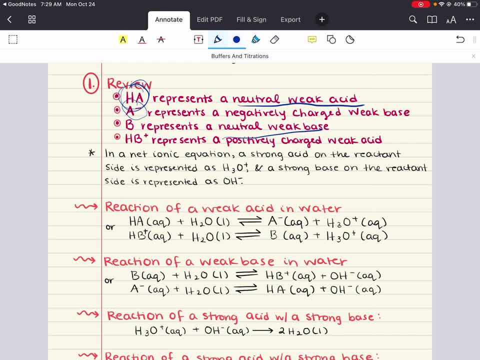 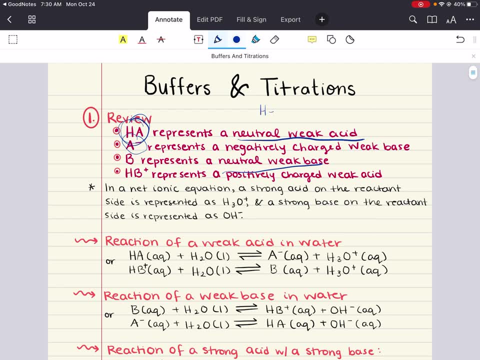 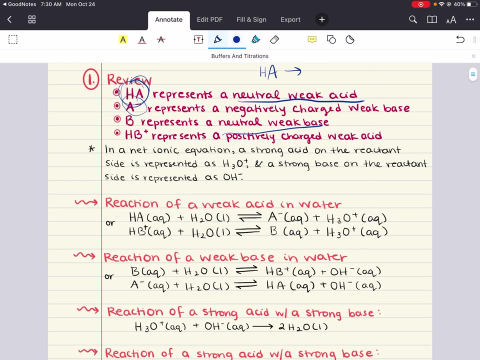 charged weak base, or in other words, the conjugate acid of the base. Alright, we've seen these before when we write out equations. Alright, acid-base reaction equations. Now, in a net ionic equation, a strong acid on the reactant side. 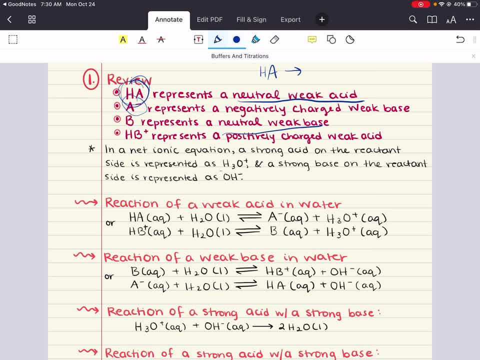 is represented as H3O+, And a strong base on the reactant side is represented as OH- Minus. In other words, okay, anytime you see H3O+, anytime you see this on the reactant side, you know this represents a strong acid. Alright, 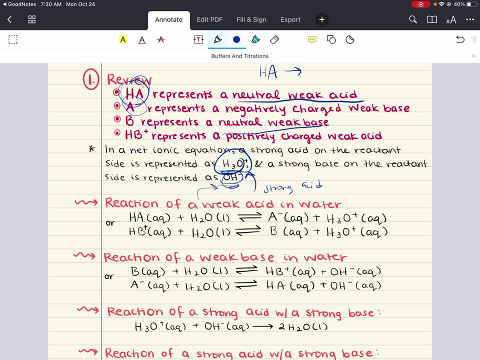 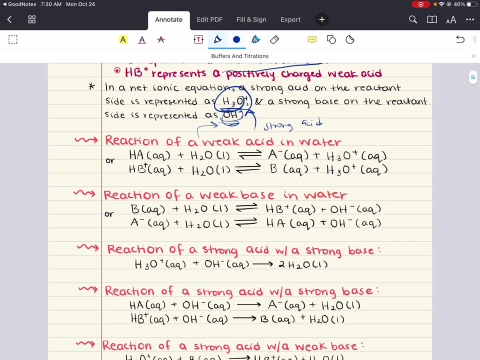 anytime you see this OH-, this hydroxide ion, alright on the reactant side, strong base, And if you remember from also the previous lectures, we reviewed the reactions we can see and how they look, how their net ionic reactions look, For example, reactions of a weak acid in. 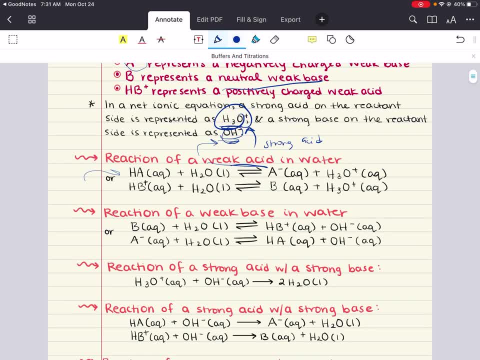 something like this, right? you'd have HA plus H2O, results in H- plus H3O+ or you can see it, HB+, right? you have your positively charged weak acid plus water equals base and H3O+. So we've seen. 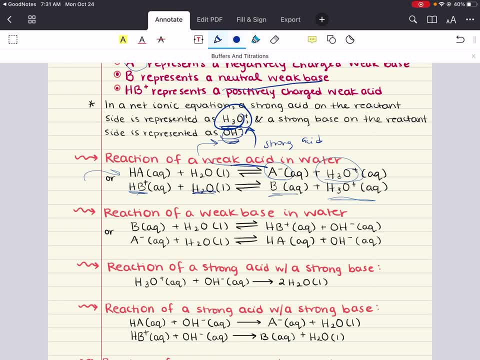 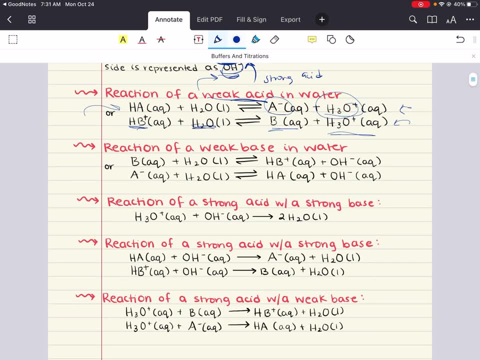 these formats of reactions previously in the last few lectures. Reactions of weak acids in water: This is what their net ionic reactions look like. Reactions of a weak acid in water: This is what their net ionic reactions look like. Reactions of a weak acid in water: This is what their net ionic reactions look like. 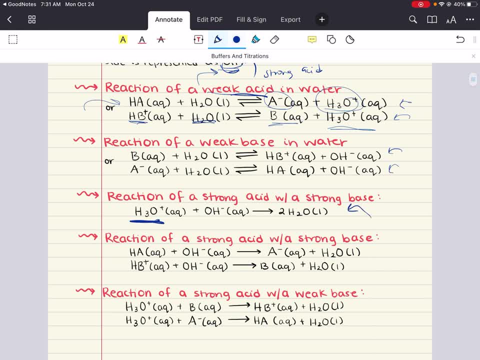 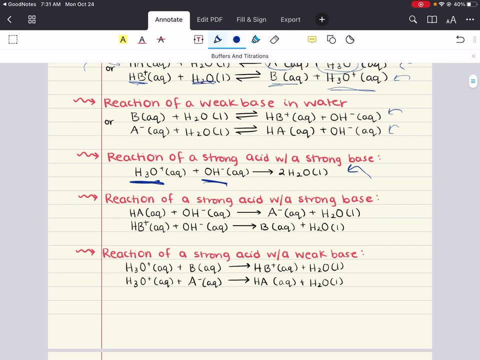 Reactions of a strong acid with a strong base. Notice how you have a strong acid and a strong base in the reactant side. Reactions of a strong acid with a strong base can also look like: look like this Weak acid. I'm so sorry this should be weak acid. 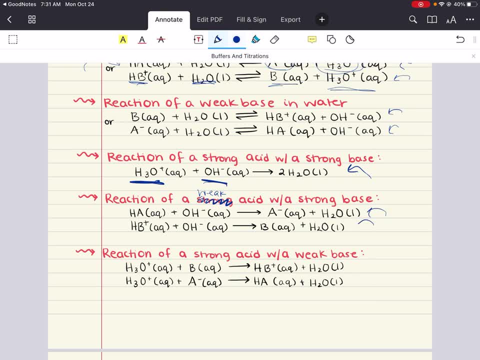 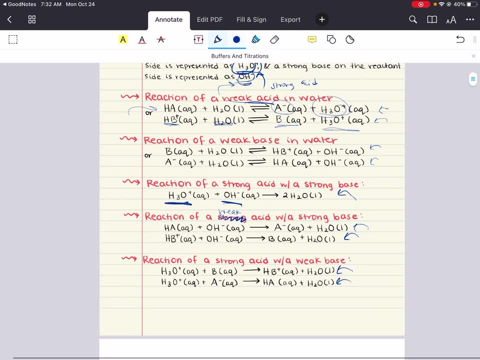 Reactions of a weak acid with a strong base: Their net ionic reactions look like this: their net ionic reactions look like this. and reactions of a strong acid with a strong base: their net ionic reactions like this. We've covered all these in details in the previous lectures. 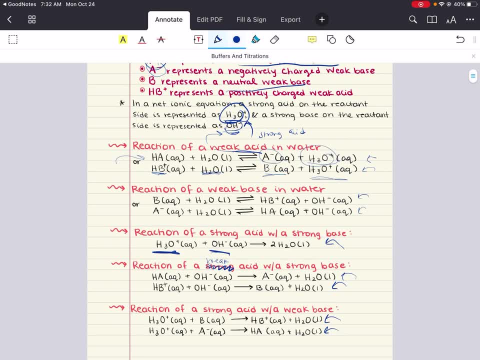 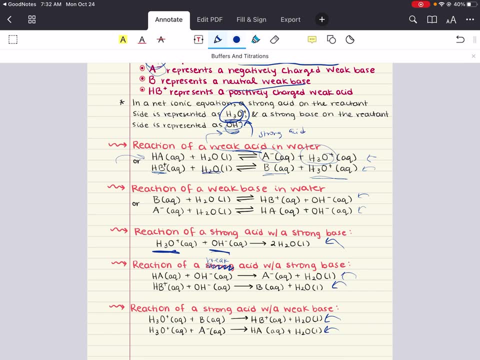 but I wanted to have a page that summarizes that for you, So this is what I've provided here in this first page: Simply a review of all the content we have dived into in depth previously. Now, once you've identified the equation that best describes the chemistry of your solution, 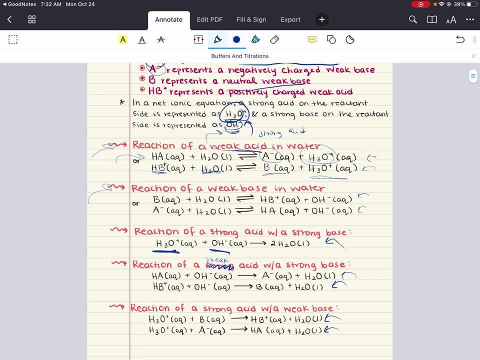 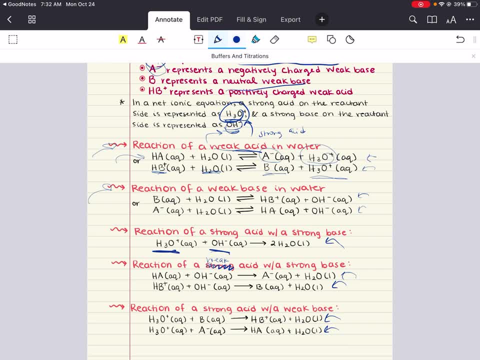 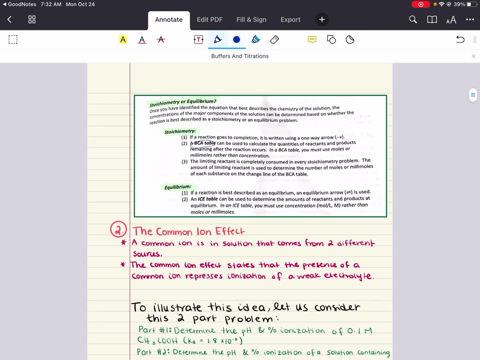 can be determined based on whether the reaction is best described by stoichiometry or by equilibrium. If it's a stoichiometry problem, all right. if it's a stoichiometry problem, all right. you're going to use a BCA table, All right. 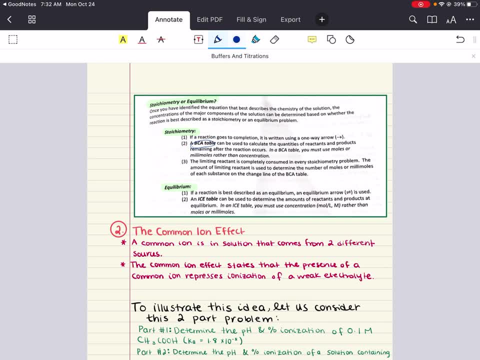 Now, this is something we haven't covered yet but we're going to cover in this chapter, so you know to use it All right, But if it's an equilibrium problem, you're going to use an ICE table And we've done many ICE tables before. where I stands for initial, C stands for change and E stands. 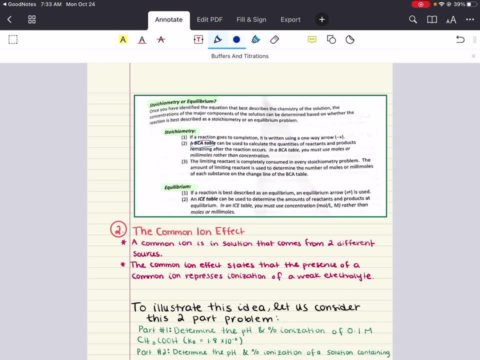 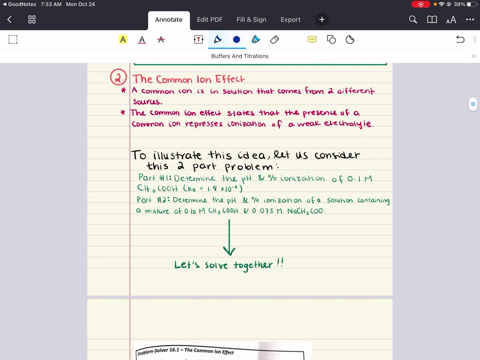 for equilibrium. We've done these previously. What we haven't done are BCA tables, but that's going to be a topic that we cover this chapter. All right. Now, with the review out of the way, let's start discussing some of the new content for this chapter. All right, And we're going to. 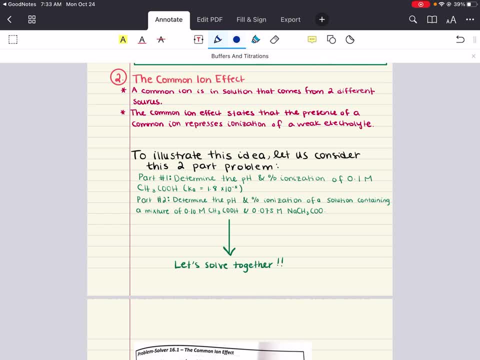 start with the common ion effect. We've seen that a system at equilibrium- all right, a system in equilibrium follows Lee-Châtelier's principle. So what that means is a weak acid at equilibrium will respond to the addition of a soluble salt that has an ion in common with the weak acid. 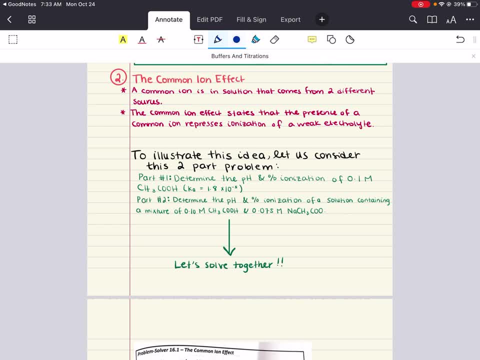 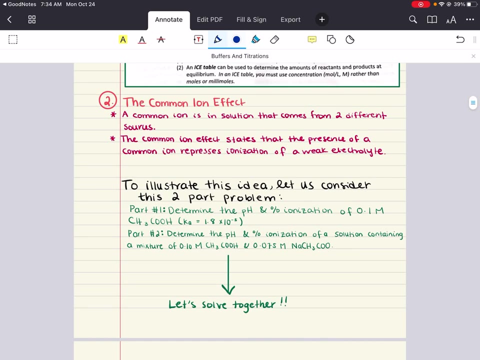 All right. For example, adding sodium acetate to a solution of acetic acid all right- is going to shift the equilibrium to the left and decrease the ionization of acetic acid. Let's look at this. All right, Let's write this down: CH3COOH plus H2O. All right, Equilibrium arrows- CH3COOH. 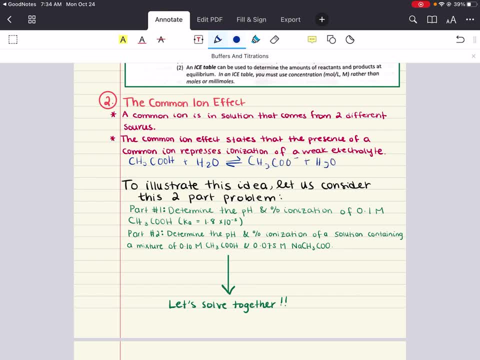 CH3COOH minus plus H3O plus- This is a three. This is also a three- Fantastic. So if you have this reaction, all right, and you decide you want to add sodium acetate to this solution, after all right, it's an equilibrium. And now you've decided you want to add some. 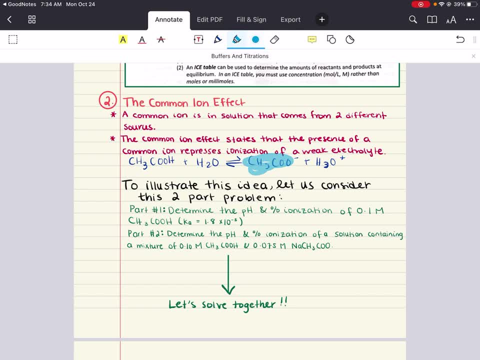 sodium acetate. all right to the solution. that's already that equilibrium. Well, now you're adding something. All right, You're adding something. You're adding more products. Okay, You want this to reach re-equilibrate again, You're going to. 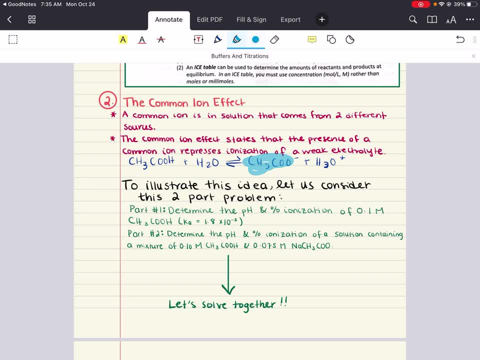 shift the equilibrium to the left. now It's going to start forming more reactants to reach that equilibrium And that's going to decrease the ionization of your acetic acid in your reactants. because now you've been adding more products, Your equilibrium is going to shift to the reactants, All right. So since your sodium acetate, 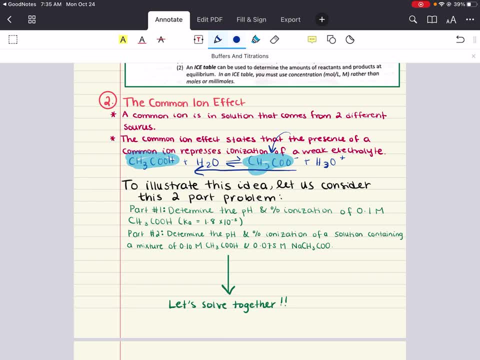 comes from two different sources in the mixture it's referred to as a common ion, And the common ion effect states that the presence of a common ion is going to repress ionization of a weak electrolyte. So what you can say is: 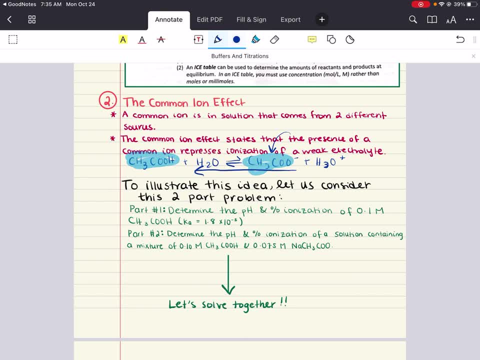 a common ion is an ion in solution that comes from two different sources, All right. So, for example, if you have a weak acid that's mixed with its salt, the conjugate base of the weak acid is considered the common ion because it comes from both the weak acid and its salt. All right, 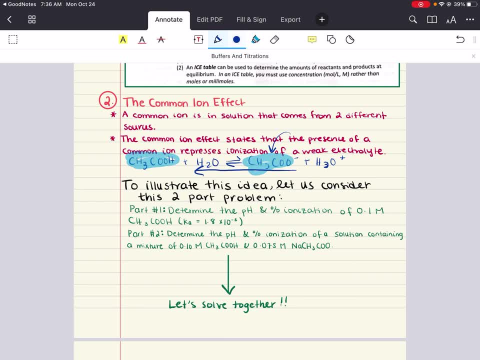 The common ion effect is an application of Lee-Châtelier's principle that says the presence of a common ion represses the ionization of the weak electrolyte. Now we're going to understand this really well by working through this two-part problem together. All right, This two-part problem. 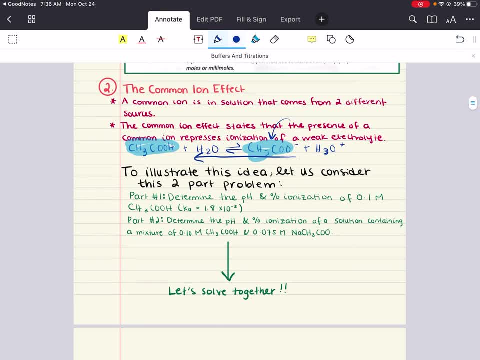 says the following. Part A says: determine the pH and the percent ionizations of 0.1 molar acetic acid. And they've given us the pH and the percent ionization of 0.1 molar acetic acid, And they've given us the pH and the percent ionization of 0.1 molar acetic acid. And they've given us the pH and the percent ionization of 0.1 molar acetic acid And they've given us the Ka value for acetic acid. 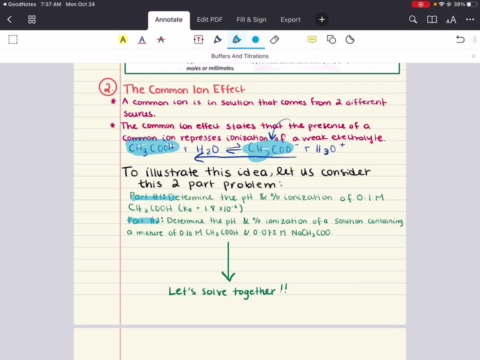 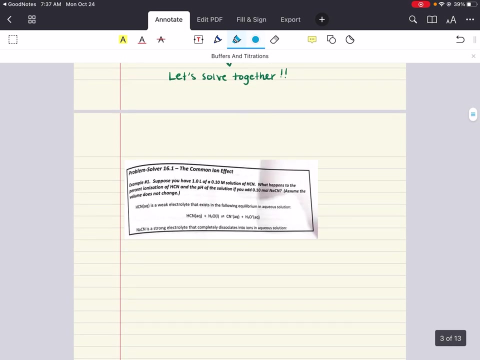 Part two says: determine the pH and the percent ionization of a solution containing a mixture of 0.1 molar acetic acid and 0.075 molar sodium acetate. Fantastic, We're going to solve this together. All right, We're going to solve this together. Let's find a blank space. We're going. 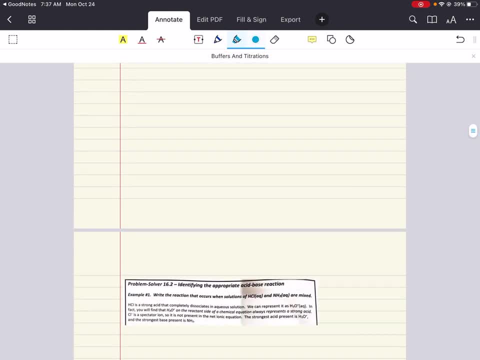 to work here and then we're going to erase it to do more practice problems. Apparently, I didn't put in an empty page for us to do that, All right, So we're going to work it here, All right, We're. 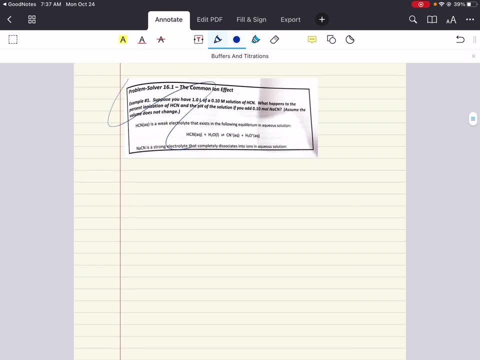 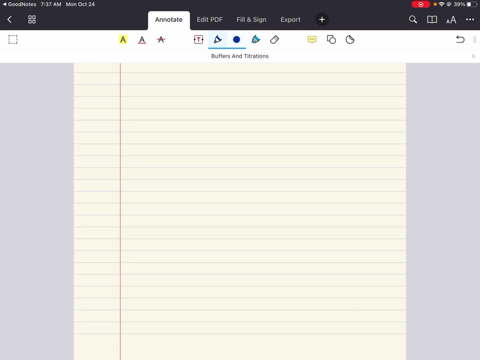 going to work our two-part problem here. We're going to ignore this for now. We're going to do it. We're going to come back to it, But we're going to use this page to do this two-part problem. we just read Now for part one. if we want to determine the pH of the 0.1 molar acetic acid, 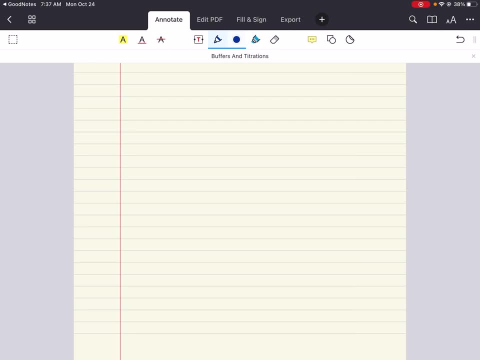 we're going to follow the same procedure. We're going to use this page to do this two-part problem. This approach we've learned in the previous chapter. All right, We're going to write HA for acetic acid, because acetic acid is not a strong acid. It's not one of the seven strong acids we. 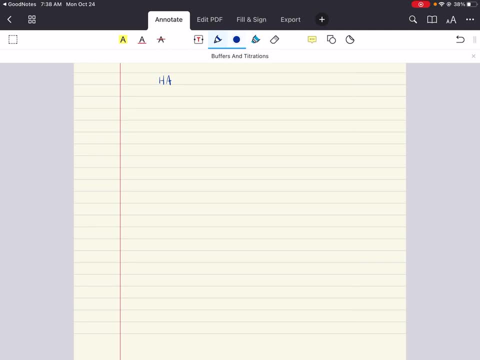 were supposed to memorize. It is a weak acid, So instead of writing acetic acid, we're going to write HA for weak acid plus H2O. All right, And that's going to form A minus plus H3O plus All. 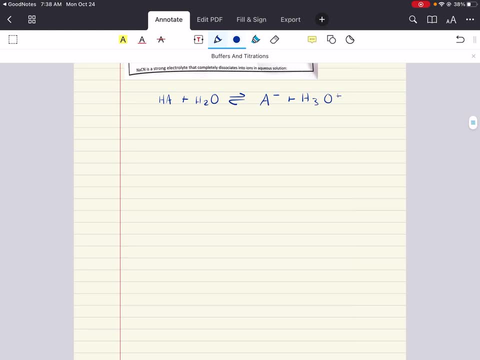 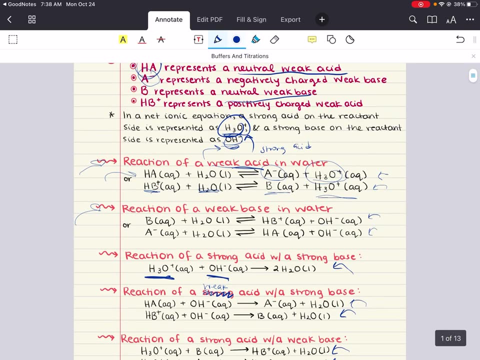 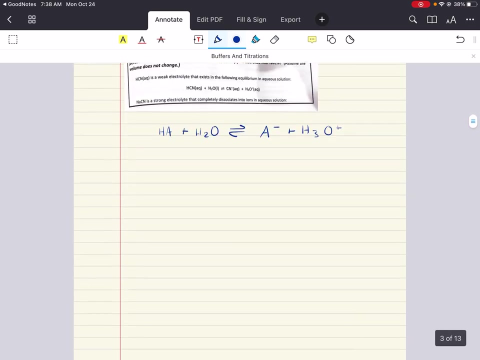 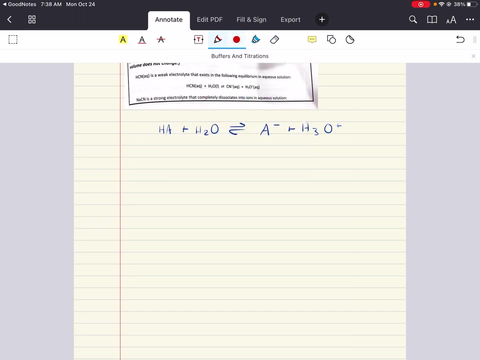 right. So that's exactly what we have done here. We have written our reaction. Now we're going to carry out an ICE table, All right, So that we can begin to solve this problem Now. initial, Initially, we start with 0.1 molar acetic acid and nothing of the others, All right. 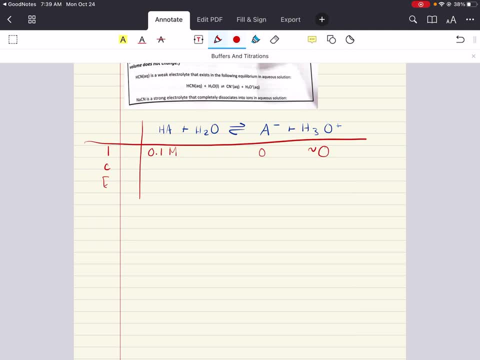 About zero. Okay, Fantastic. Now what's changing? Well, we're going to lose some reactants to form products. All right, Awesome. And now for the equilibrium. we can write 0.1 minus X, And then we can write X here and X. 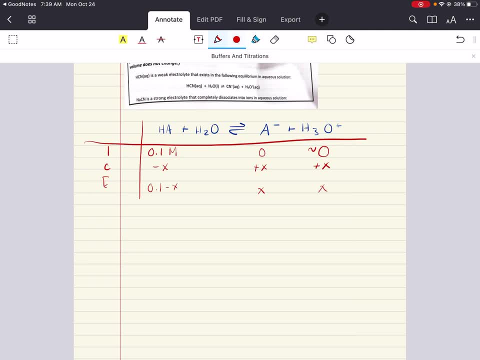 Here. Now notice that we're going to assume that this is really just approximately 0.1.. Remember our 5% rule. We're going to make this assumption that it fits this 5% rule and we can approximate 0.1 minus X to just 0.1.. Now the next step is to insert the equilibrium. 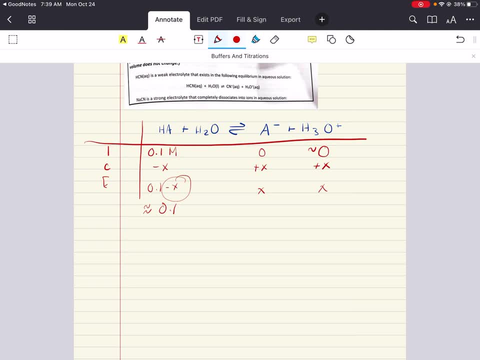 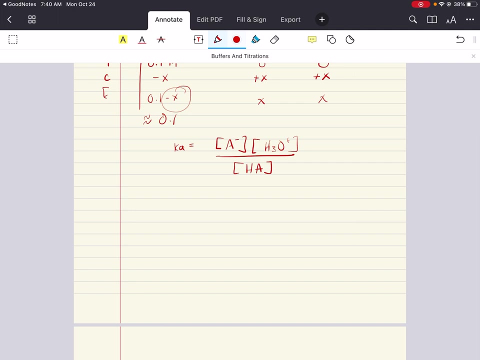 values Into our KA equation. All right, Now, if you remember, our KA equation is going to be product over reactants. All right, Fantastic, We know what our KA value is. They've given it to us. They told us: hey, the KA value for acetic acid is 1.8 times 10 to the minus. 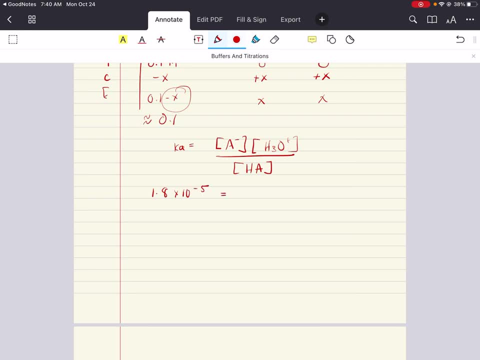 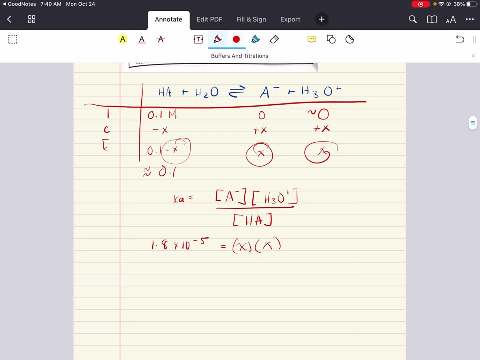 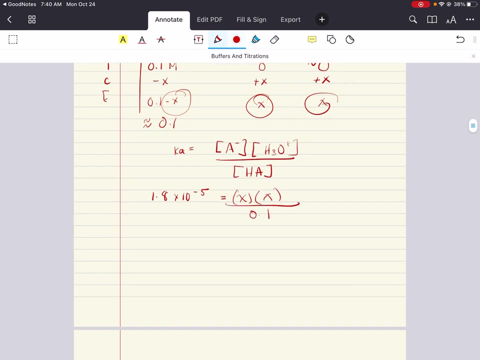 All right, So we can plug that in For A. we're going to plug in X here and then another X here. All right, Because this is what we've defined to be our equilibrium status for the product: X, and X over 0.1 for our reactants. All right, This is just an essentially X squared over. 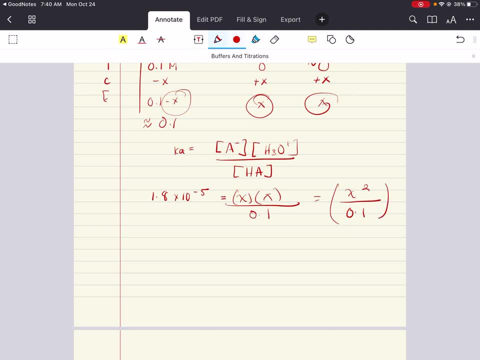 0.1.. All right, Now we can multiply both sides by 0.1 to cancel that out. All right, 0.1.. And then, in addition to that, we can square root both sides so that we can get our definition for. 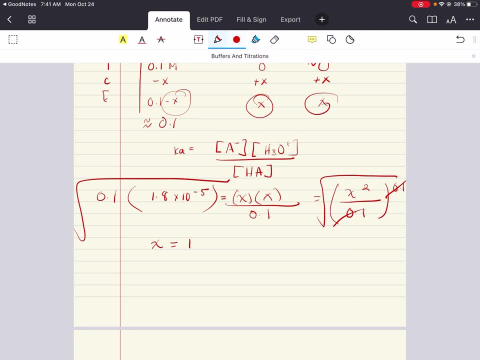 just X. If we do all that, X is just 1.34 times 10 to the minus 3.. That means our H3O plus concentration is equal to X, which is just 1.34 times 10 to the minus 3.. And this is the same for. 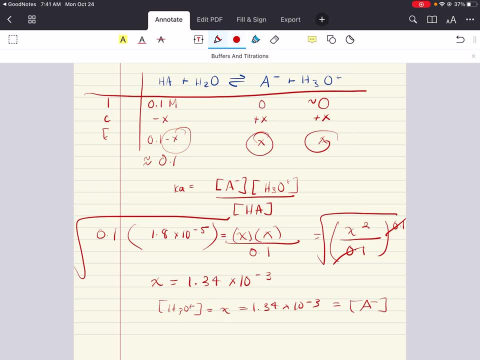 our conjugate base A minus. All right, Now we're not done yet. What did they ask us for? They asked us for the pH. All right, If you remember from our previous chapter, our pH, we can define this by just. 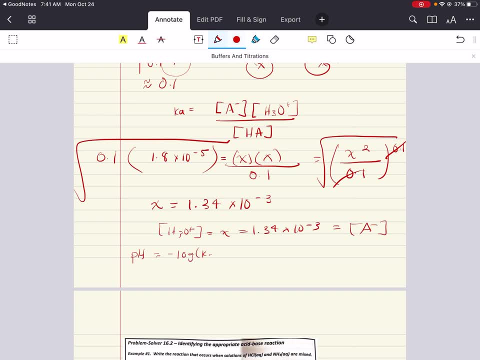 doing the negative log of our KA value. Oh, I'm sorry, Not our KA value, Our H3O plus value, All right, I'm so sorry about that. So if we take the negative log of our H3O plus, 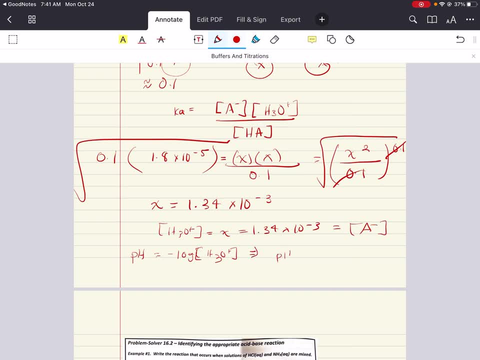 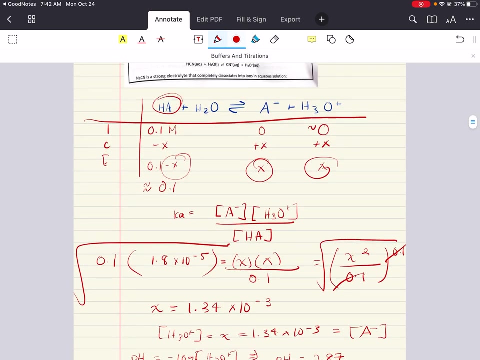 what we're going to get for our pH now is that pH is equal to 2.87.. Now, still again, we are not done. They asked us to determine the pH and the percent ionization. All right, To determine the percent ionization, we're going to divide the amount of acid HA, so acetic acid, all right. 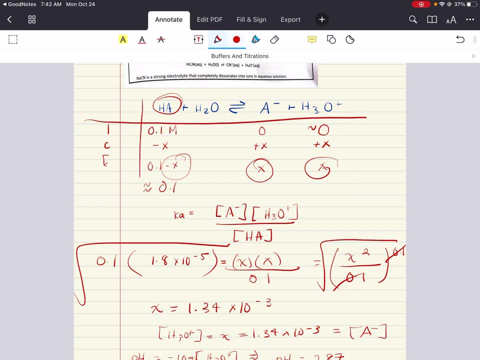 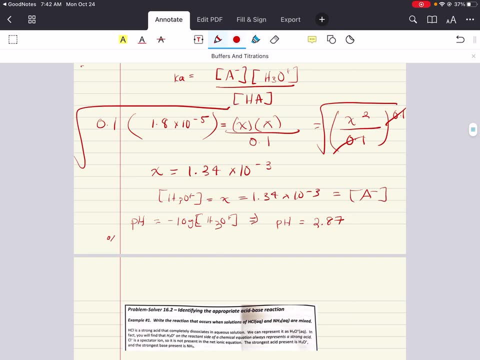 that ionized by the initial concentration of HA. All right. So what that means is for percent ionization. I'm going to write it down here: percent ionization. All right, We're going to do this. X over 0.1 times 100%, We're X. 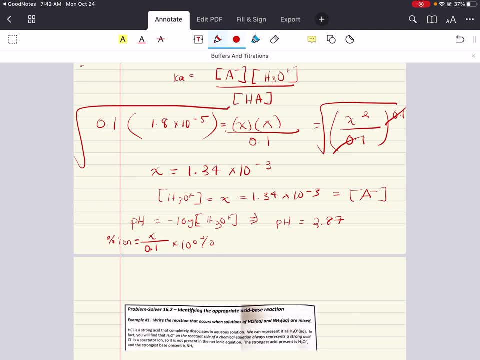 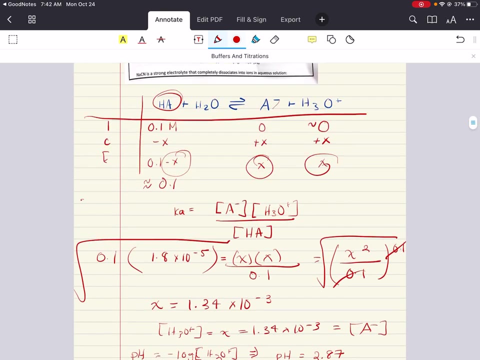 all right, We're going to divide the amount of HA that ionized by the initial concentration. Well, the amount of the acetic acid that ionized, all right, is just 1.34 times 10, to the minus 3, right. It ionized to form its conjugate base and we determined what X was. 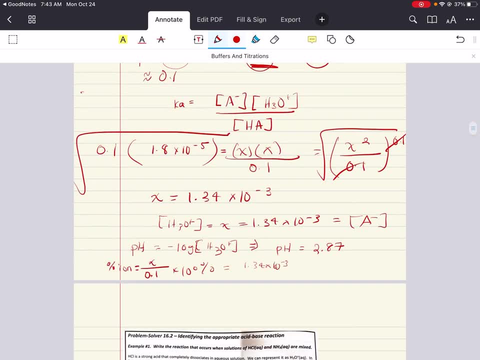 X was 1.34 times 10 to the minus 3.. All right, And then we're going to divide that by the final amount. all right, the initial concentration of HA, which was 0.1,. all right, and then multiply. 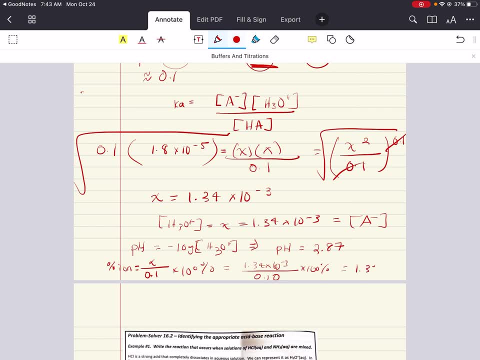 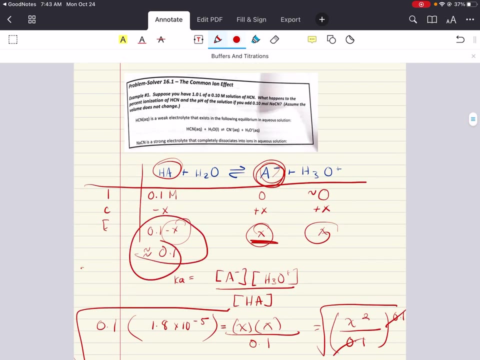 by 100% And what we get is 1.3%. The value of X here is less than 5%. So guess what? That reaffirms that our approximation in the first column here was appropriate as well, so that we got reaffirmed that this was the right move to do. 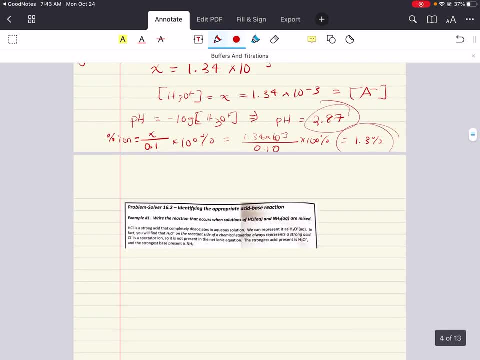 All right, And so we've done it. We found the pH 2.87.. We found the percent ionization. All right, Fantastic. Second part of this problem says: well, we need to consider, all right, a solution containing a mixture. 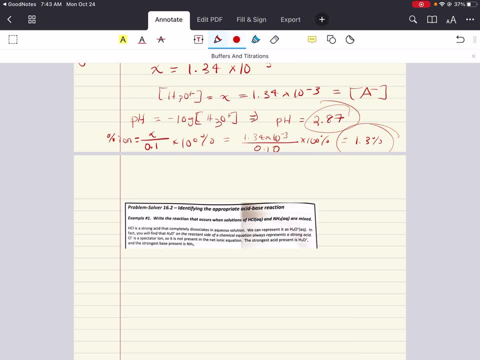 of 0.1 molar acetic acid and 0.075 molar sodium acetate. okay, Well, we're going to have to also set up an ICE table for this, where the initial concentration of A minus. guess what It's no. 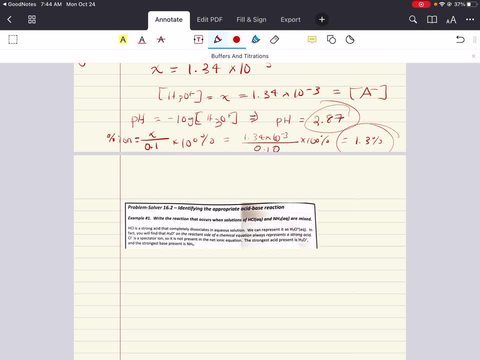 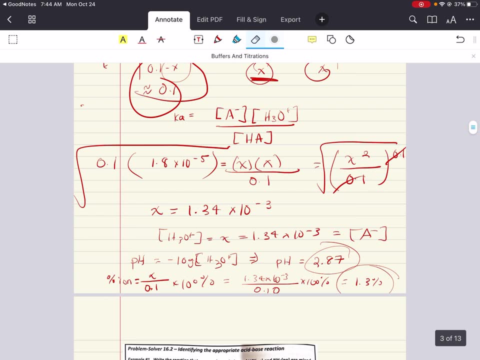 longer zero. all right, It's no longer zero. We now have 0.075 molar of A minus to start this problem off. So let's do that part, Let's erase all of this and let's do part two. All right, This is a good reminder of everything we learned in the previous chapter. 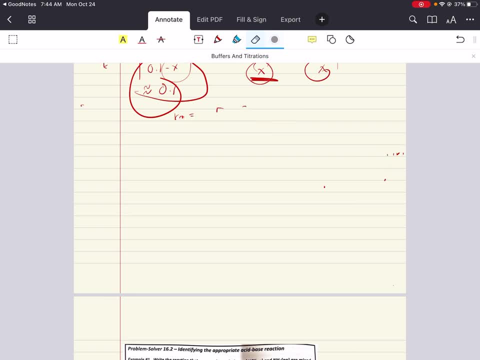 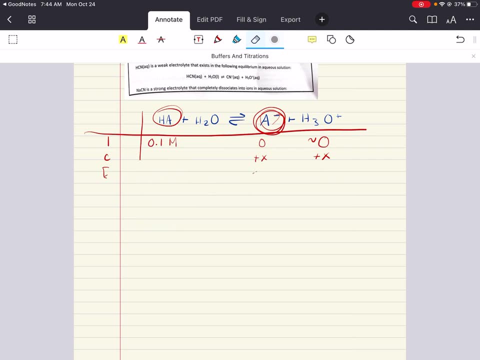 as well, All right, But now we're stepping it up a game. Now we're not going to have zero for both our products, All right. Now this is no longer zero here, because in part two, if you remember, we have 0.1 molar acetic acid. 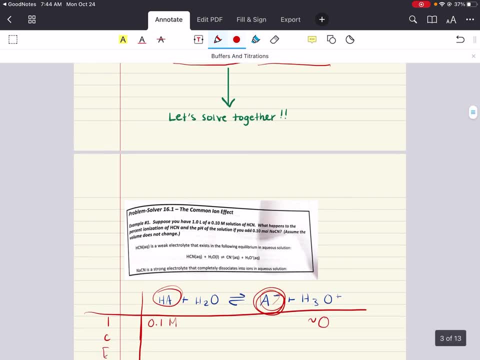 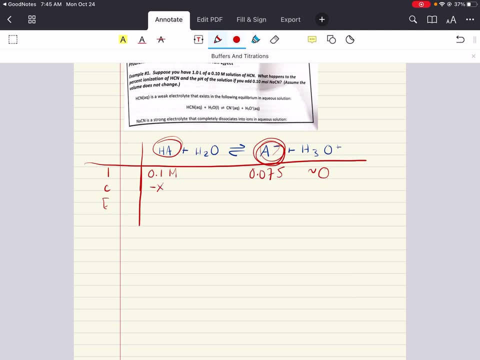 But now we also have 0.75 sodium acetate, So that is going to go here 0.75.. All right, Fantastic. We're going to lose reactants to form products And again we can write 0.1 minus X. 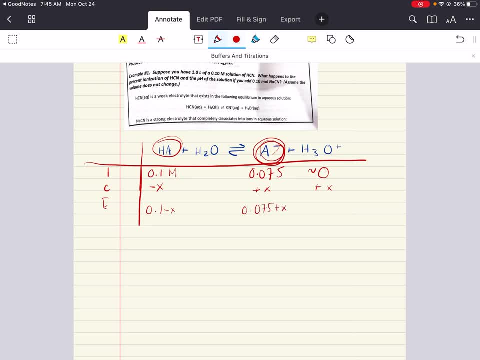 and we can also write 0.075 plus X and X over here, But we're going to assume that our 5% rule is going to follow and we're just going to get rid of this part for simplicity And, hopefully, an answer that reaffirms that we did a good job by saying that the value of X is less than 5%. 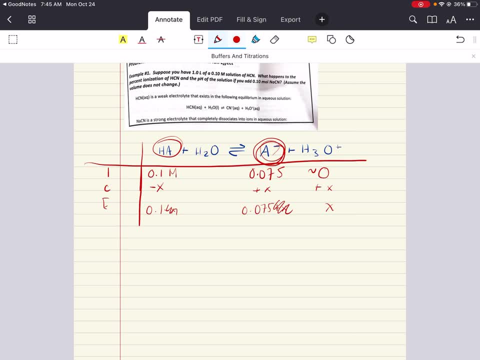 of the initial value, so we don't have to worry about it. So let's work this out. This table contains these two approximations and we're going to take that and insert the values into the KA equation, All right. So, if you remember, our KA is going to be product over reactants. 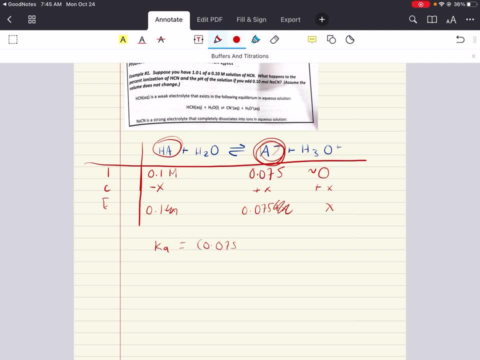 Okay, We're going to cut it short and we're just going to write 0.075 multiplied by X. Those are our, Our product over our reactants, which is 0.1.. And our KA is again the same: 1.8 times 10 to the. 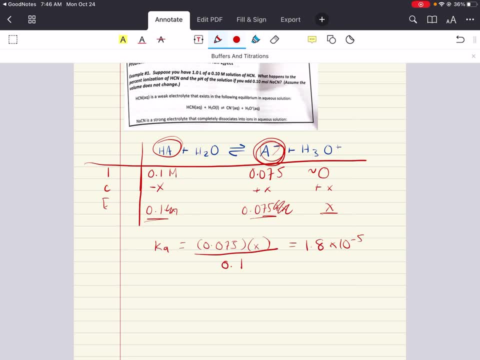 minus 5 for acetic acid. All right, What we're going to do is multiply both sides by 0.1 and divide by 0.075.. So these cancel out and this cancels out. We do the same thing on the. 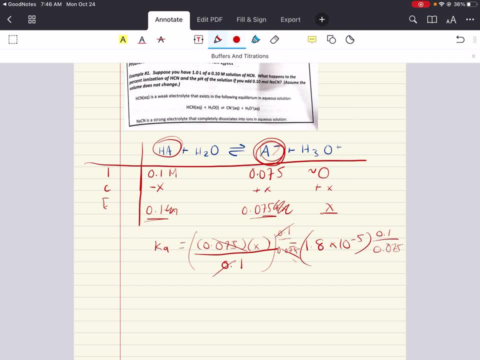 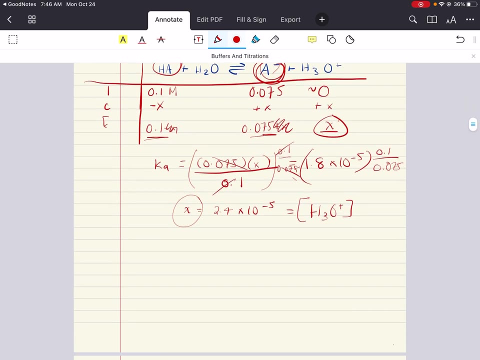 other side. All right, And now we can solve for X. X is 2.4 times 10 to the minus 5.. If this is what the value of X is, Then that is what our concentration of H3O plus is equal to, And that way we could figure out. 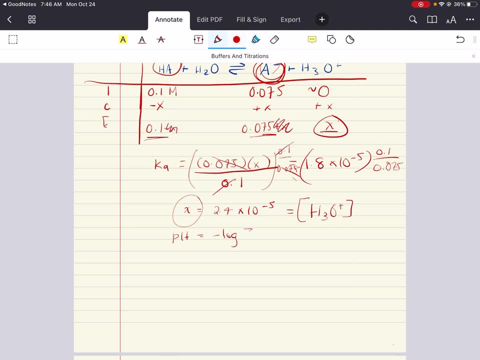 the pH again by just taking the negative log of H3, the concentration of H3O plus, which is 2.4 times 10 to the 5.. So this is going to give us a pH of 4.62.. All right, Now what about the? 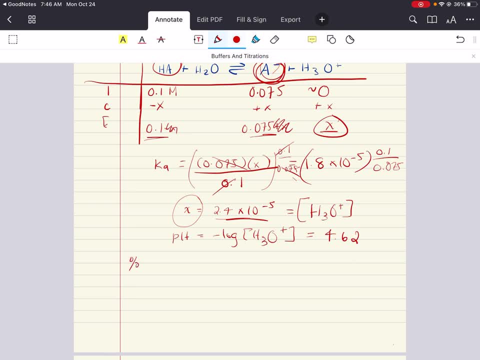 percent ionization: Again, very similar, All right, Very similar to the previous one. The percent ionization we're going to do 2.4 times 10 to the minus 5 over what we started initially with the weak acid concentration, 0.1. And then we're going to multiply this by 100%. 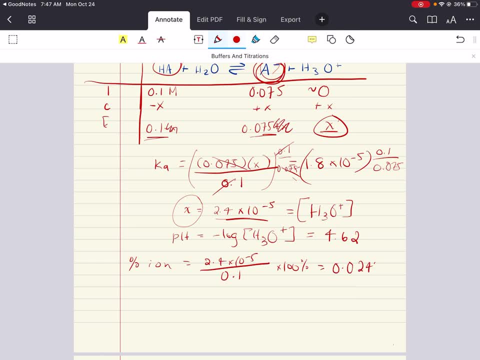 And this gives us 0.024%. That is the percent ionization. Now the value of X here was less than 5% of the initial concentration. So guess what? Our approximation was very appropriate, The most important thing to see in this example. 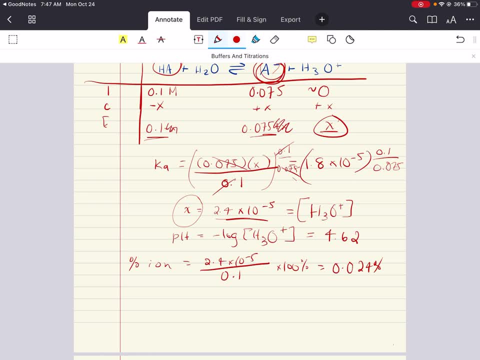 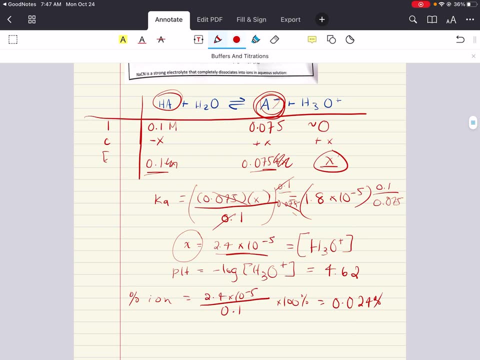 right is that the percent ionization of our weak acid, our acetic acid, in the presence of a common ion. right here, this problem we just did is much less than that. when there was no A minus to start off with, Okay, When we had. 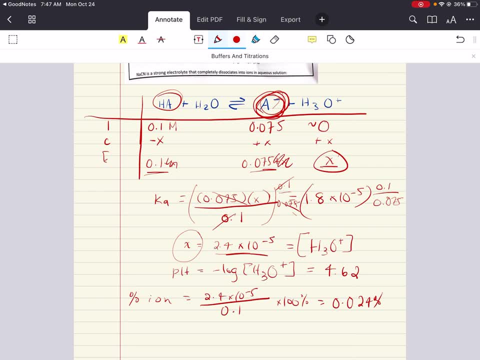 HA and A minus. to start off with our percent ionization was so much smaller. All right, This illustrates The common ion effect That presence of A minus has represented the ionization of HA, the weak acid, the acetic acid, And guess what? It resulted in a higher pH and a much lower 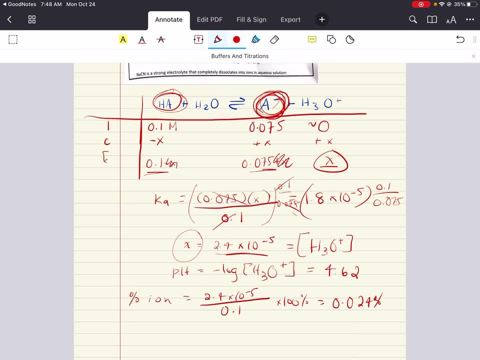 ionization, percent ionization- All right, Fantastic. So we did it. All right. We solved two problems, part one and part two. All right, And guess what? We're going to do another one now. We really want to make sure we nail this, All right. 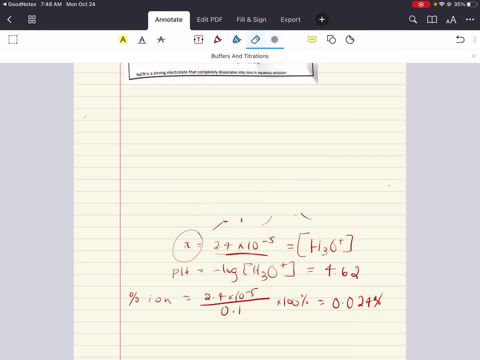 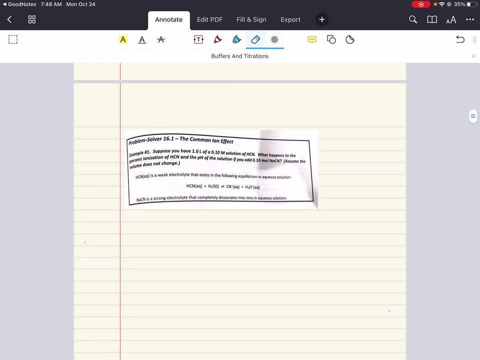 So let's look at this example problem. Let's erase all of this so we can work it out here. All right, Erase, erase, erase, Beautiful. Let's do this practice problem. Suppose you have one liter of 0.1 molar solution of HCN. What happens to the percent ionization of? 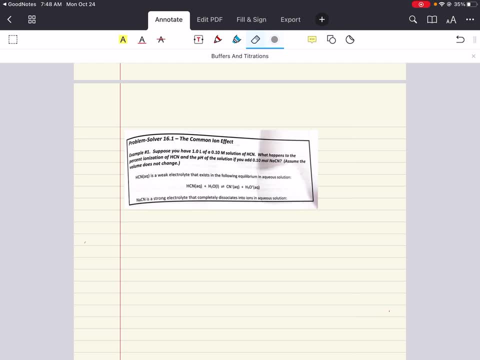 HCN and the pH of the solution. if you add 0.1 mole Sodium cyanide, All right, Cyanide, Fantastic. So HCN is a weak electrolyte. All right, It's a weak electrolyte. We can write our equation as We can write it fully like this: HCN plus H2O is 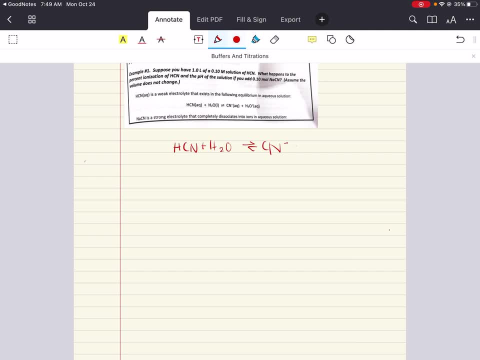 going to give us CN minus plus H3O plus- Fantastic, All right. Now, sodium HCN is a weak electrolyte. Sodium cyanide is a strong electrolyte and it completely dissociates into ions in this aqueous reaction. All right, So we can rewrite this. We can kind of view this. 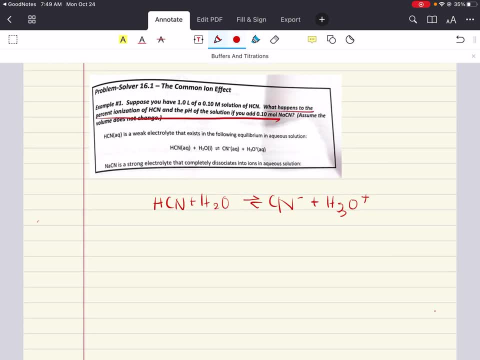 as All right. What happens to the percent ionization as we add? Okay, So let's think about this. HCN is a weak electrolyte and it exists in this following equilibrium of this in the aqueous solution, Now sodium cyanide, which gives you the CN minus. this is a strong electrolyte. It. 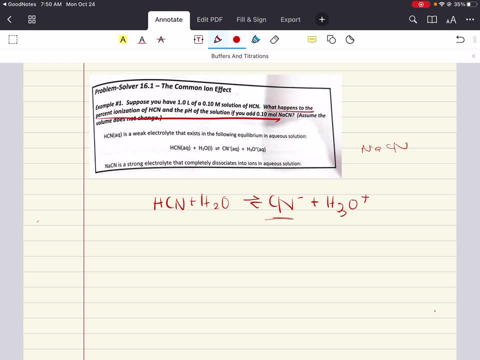 completely dissociates in aqueous solution. NACN completely dissociates into NA plus plus CN minus, which is the conjugate base. by the way, This is the conjugate base of HCN That makes for chair with iron in one side, forehand, and акne in the other right hand side's face and 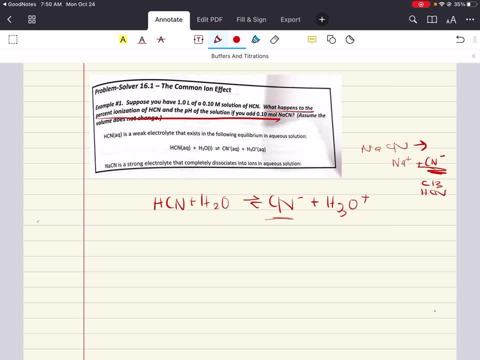 valores for exercise. So these are the similarities that we make in usingbereich and fundamentals that we do to CNA plus sodium. So that pens in for this aqueous solution. Again, it means a conjugate base. Therefore, what happens when we add sodium cyanide to? 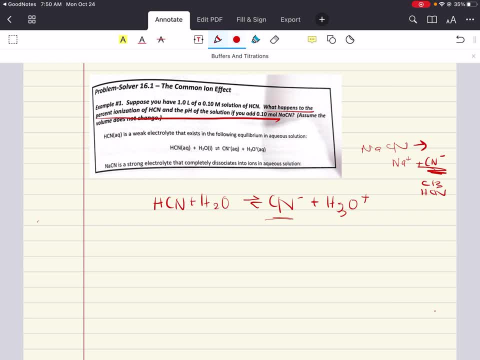 exoskeleton, H4 is taken as a common cell composition. think about hydrogen and comum soot. if this shows here the fact that 우�ست has not been CN minus is caused by the common ICON, Now tell us why aren't you able to find them? Well, there's an, however common 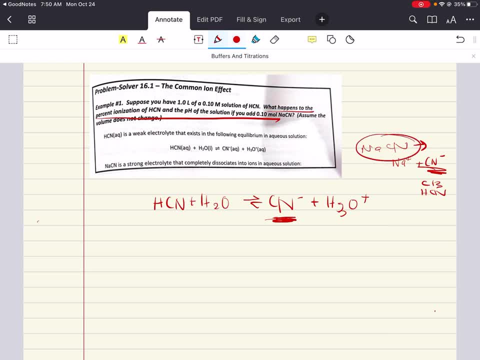 ROM here. The same thing as Sen plus Ac0 plus Ac2 plus Ac2.. You could find thoseprior called CN and CN plus monoclonal山ass as 눈ing. much less, and except for attention to people, It comes from sodium cyanide and it comes from HCN, all right. 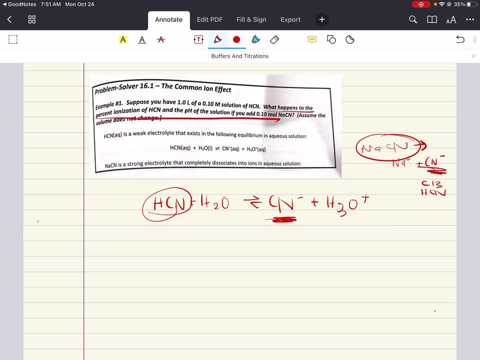 That means when we add CN minus to a solution of HCN, all right, it causes the equilibrium to shift to the left to re-equilibrate. This means that HCN is going to what Ionize less than it would If there was no CN minus additionally present. all right. 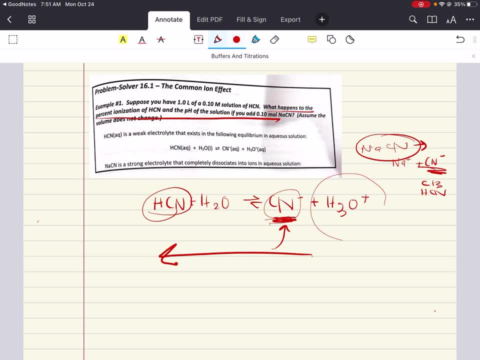 A shift to the left also means- guess what- that the concentration of H3O plus also goes down, because when you're adding CN minus, all right, this is the product it wants to re-equilibrate. It's going to move to the left. 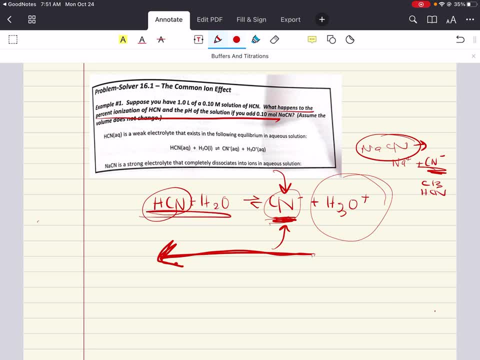 The reaction is going to move to the left to now form more products instead, all right, Which means we have less products overall. That means we have less H3O plus. When we have less H3O plus, all right, the pH goes up. 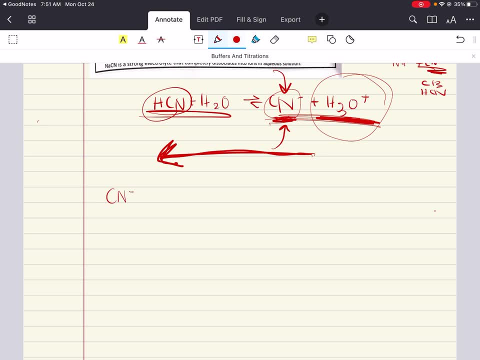 So what we've determined is that CN minus is the common ion, because it appears both here in HCN and over here as the thing that has dissociated from sodium cyanide. all right, We've determined that. all right. So CN minus is the common ion. 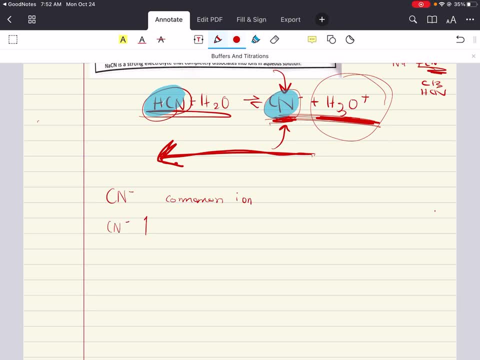 If we add more CN minus, all right. we add more, all right. equilibrium will shift to the left. If it shifts to the left, all right. what are you going to have more of? You're going to have more HCN, all right. 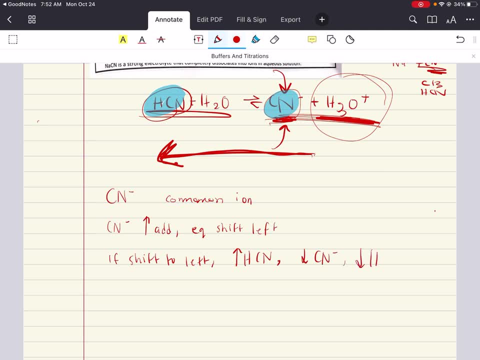 You're going to have less CN minus, less H3O plus being formed. If you have less H3O plus being formed, all right, Your pH. Your pH goes up, all right, Fantastic. So these are all the important points for you to take away. 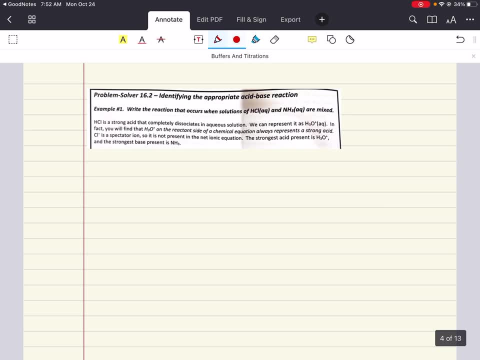 Now this other problem here I am going to let you figure out. with everything that we've learned so far, you should be able to solve this problem. Let me know what you get in the comments below and we can talk about it all right. 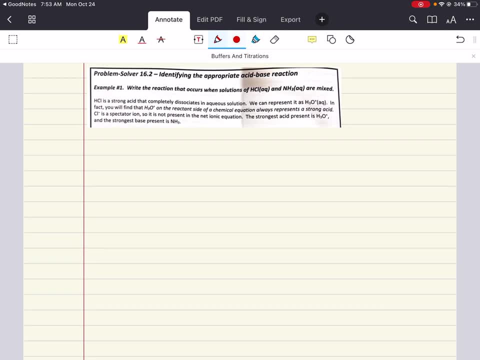 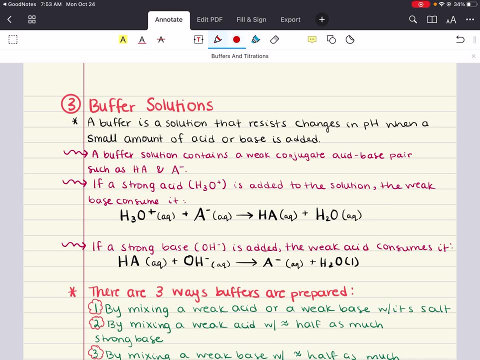 Fantastic, Let's see All right. So let's move on The next topic that we want to cover in this chapter. that's very important. all right are buffers and buffer solutions. all right, This is going to be very important. 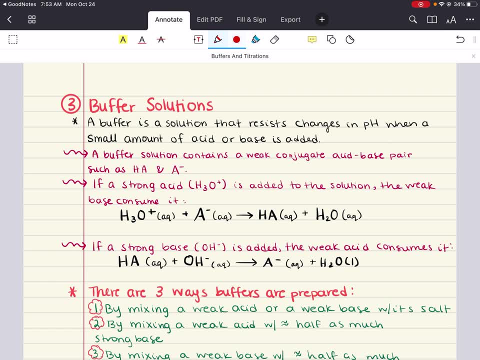 So let us define: a buffer solution is a solution that resists changes in the pH when a small amount of acid or base is added. So you can think of Of a solution that you might have that is at a specific pH that you want it to be all. 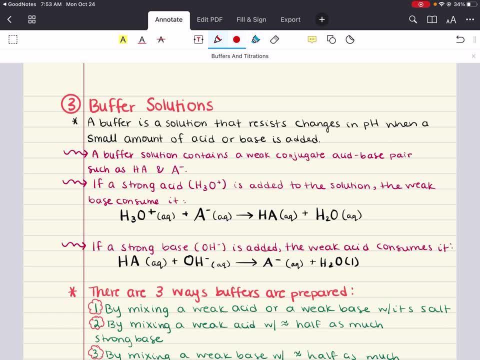 right. If you have a buffer system in play in the solution, any small amount of acid or base that you may add to it is not going to affect it because of the buffer solution. So the buffer solution is a solution that resists that change in pH whenever a small 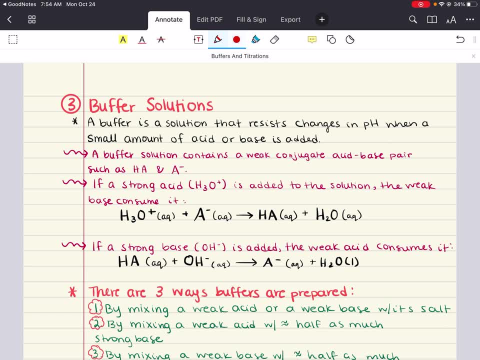 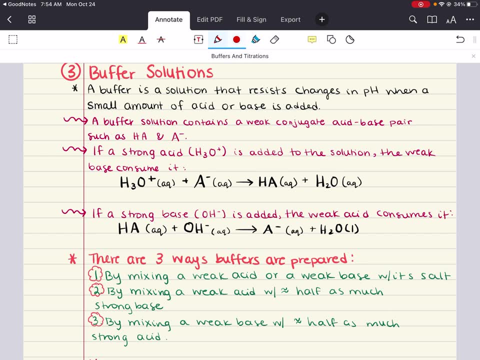 amount of acid Or base is added. Now, a buffer solution contains a weak conjugate acid base. pair right Something like HA, a weak acid or a minus. all right, If a strong acid is added to the solution, then the weak base consumes it. 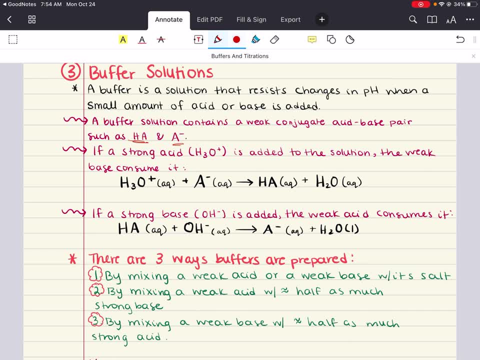 If a strong base is added, then the weak acid consumes it, And that way you can resist changes in the pH. Now, in both cases, the pH does not change very much because the strong acid or strong base is consumed by the buffer. So let's motivate this. 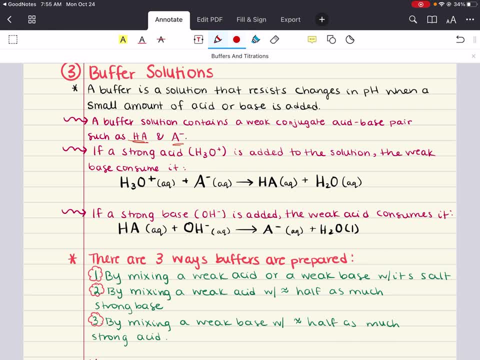 Let's motivate this buffer solutions conversations by saying: how much will the pH change? All right, How much will the pH change If We add, If the same amount of hydrochloric acid is added to a one liter, one liter of a buffer? 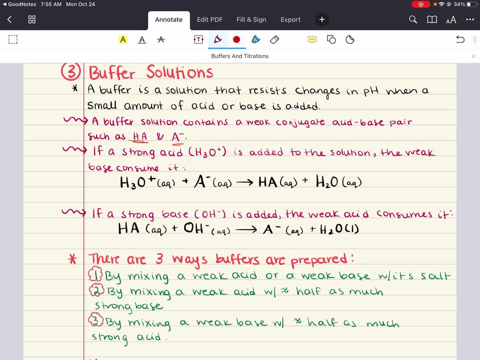 containing 0.1 molar acetic acid and 0.1 molar sodium acetate. All right, So let me start here before we do that: adding a small amount of strong acid or strong base to a unbuffered, I believe. 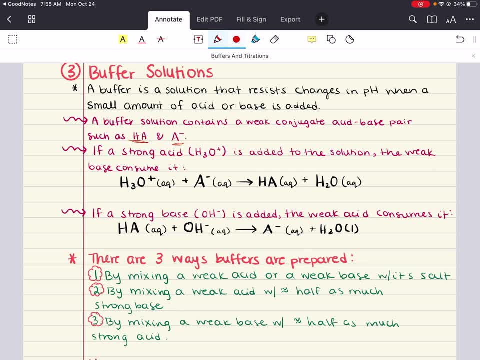 A pure, unbuffered water. What is going to? what was going to happen? That's going to result in a dramatic change in pH. For example, consider the pH change that would happen if 0.01 mole- all right. what would? 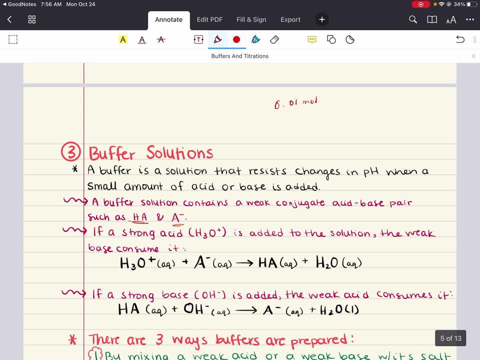 happen if we took 0.01 mole- all right- of HCL and we added that to one liter of just pure HTL? All right, Before adding the acid? the pH is just going to be your normal pH of water, right? 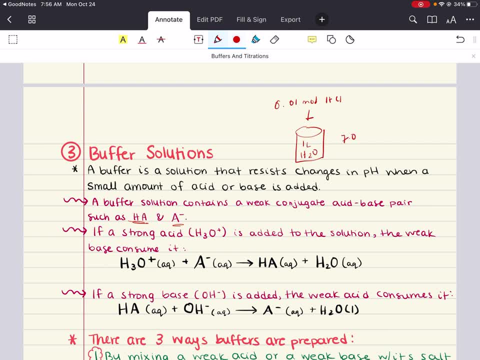 Seven, seven pH. All right. If you add this HCL to the water- just the water- the new concentration of H3O plus would be equal to that of the HCL that's added. it'll be 0.01.. 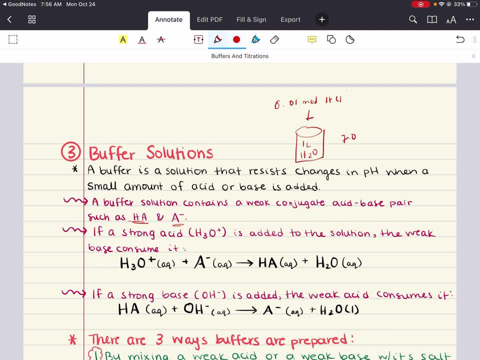 That's going to result in a pH change of this water by adding this amount of hydrochloric acid To two. All right, So that means adding even that small amount of moles of hydrochloric acid: 0.01 mole of. 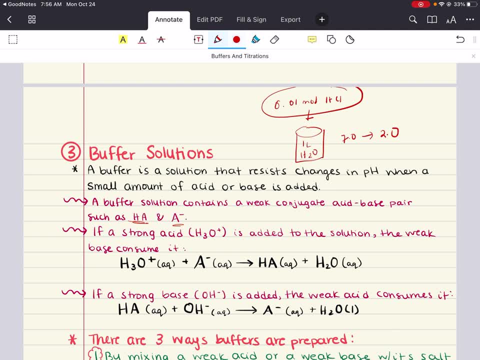 hydrochloric acid to pure water is going to cause that pH to plunge. I mean, look at that difference going from seven pH to two. That is a very dramatic change. And also keep in mind, by the way, that the pH scale is a log based scale. 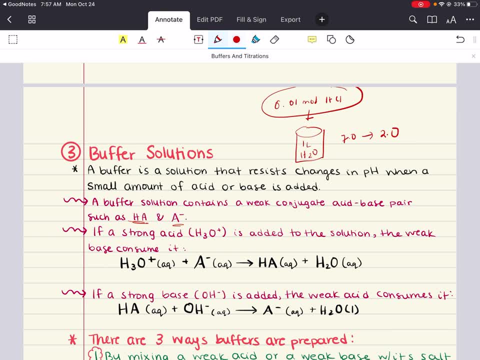 So that means each unit. It corresponds to a power of 10.. That means going from seven to six corresponds to a power of 10. going from seven to five, That's 10,, 10,, 10 times 10.. That's a hundred. 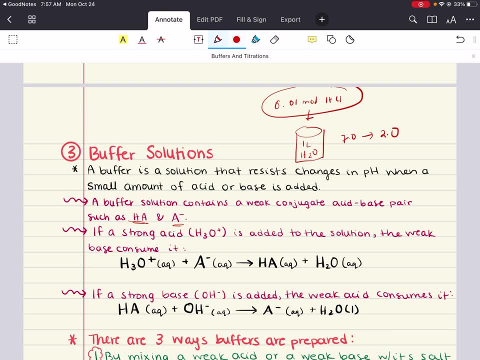 That's a magnitude of a hundred. going from seven to five, going from seven to two, That's a hundred thousand times greater than it was before the acid was added. All right now. in contrast, how much will the pH change If that same amount of HCL 0.01 is added to one liter of a buffer? all right, if we 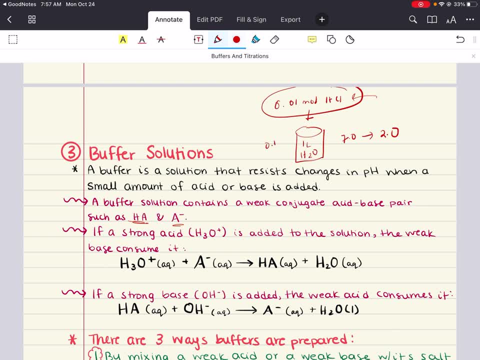 add this to a buffer, like what we like what we did previously: 0.1 mole acetic acid and 0.1 mole- or molar, sorry- of sodium acetate. H3CO minus. All right If you add 0.01.. 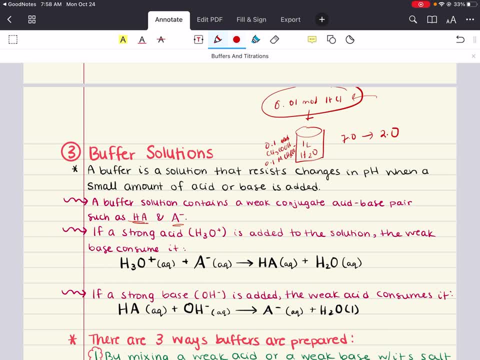 0.01.. 0.01.. 0.01. 0.01.. 0.01 moles of HCL to this system, How will the pH change? Well, to answer this question, we're going to begin by calculating the pH of the solution. 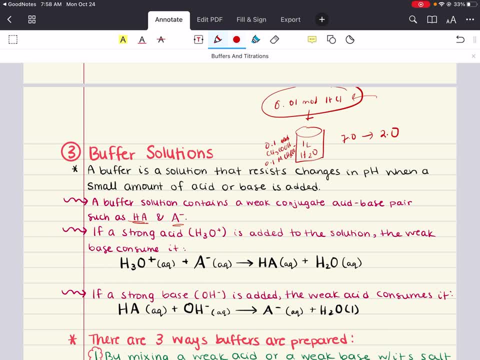 before adding the acid. All right, And similar amounts of weak acid and it's weak conjugate pace are present here. All right, Since, since there's no strong acid or base initially, we're going to describe this reaction using an equilibrium ice table. 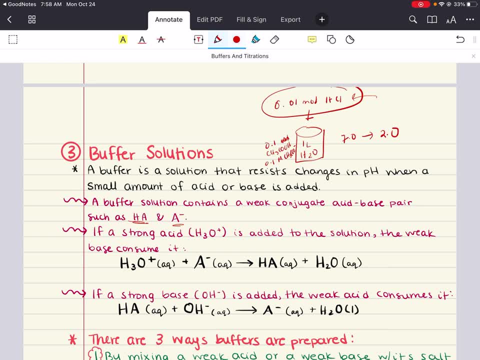 So that's what we're going to start with. All right, Did I leave room to do this together? Yes, I did. All right, I left room for us to do this. And here's the problem, right, And apparently I forgot. 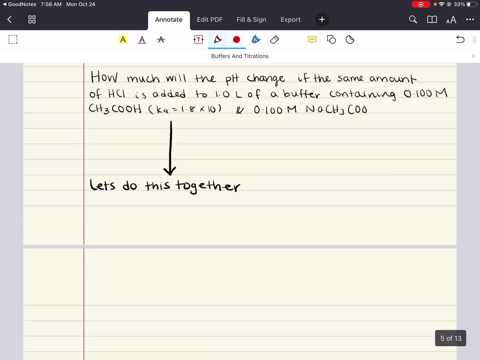 How much will the pH change if the same amount of HCL, which for our unfiltered water was 0.01 mole, is added to one liter of a buffer containing the following: Let's do this together, All right. Let's start by writing: HA plus H2O. 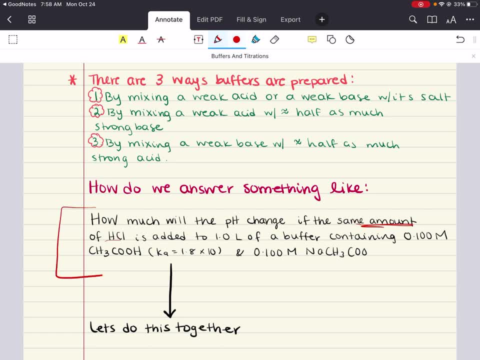 H2O equals 0.01.. All right, Let's do this together. All right, Let's start by writing HA plus H2O: H2O equals 0.01.. All right, Let's do this together, All right. 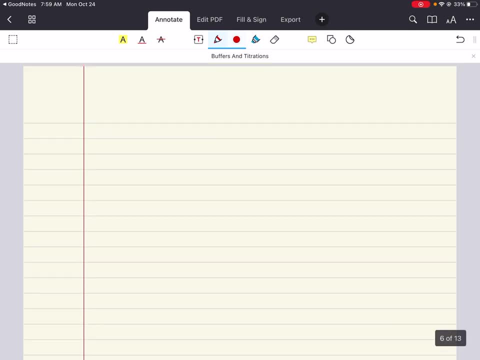 Let's start by writing HA plus H2O: H2O equals 0.01.. All right, Let's do this together. Let's start by writing HA plus H2O: H2O equals 0.01.. All right. 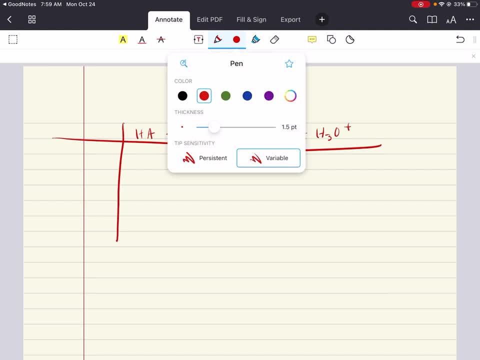 Let's start by writing HA plus H2O. All right, Let's start by writing HA plus H2O. H2O equals 0.01.. All right, Let's start by writing HA plus H2O. We're going to use the equilibrium arrows: a minus plus H3O plus. 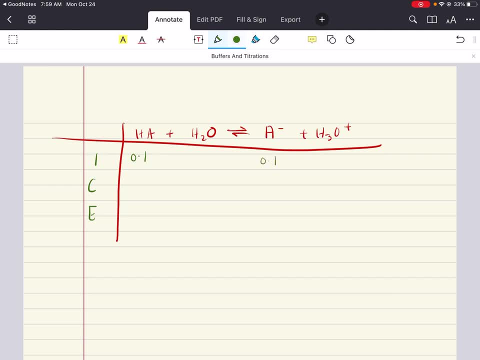 All right, Let's write our ICE table: ICE initial: 0.1.. All right, 0.1 and approximately zero. We lose reactants to form products in 0.1.. We're going to assume that the minus X is very negligible. 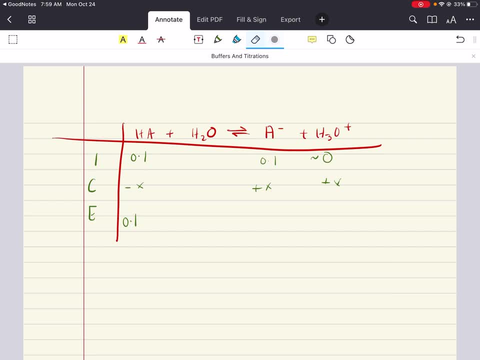 So we can ignore that it is 5% less, that it's at least 5% less, All right, than the concentrations of these, all right. and then same thing goes for a minus. we're going to assume the plus x is um follows the five percent rule and we can, we can lose it, all right, so that 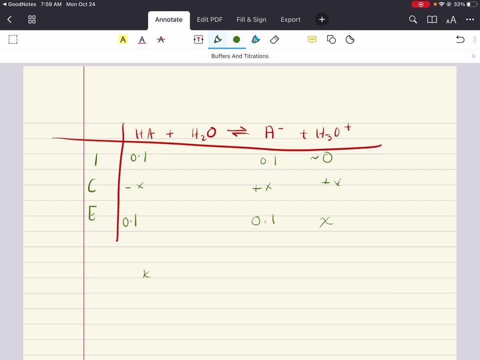 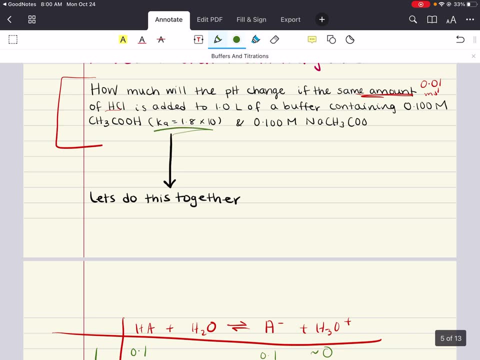 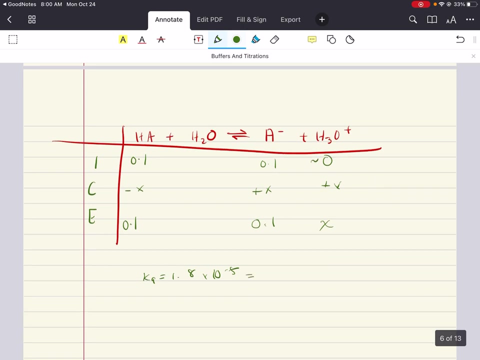 we have the following now. fantastic, now we know the ka here. the ka is 1.8 times 10 to the minus five. they give it to us right here. all right, 10 to the minus five, beautiful, all right, let's solve the ka. it is re a product over reactants, so 0.1 times x over reactants, 0.1, all right. essentially, 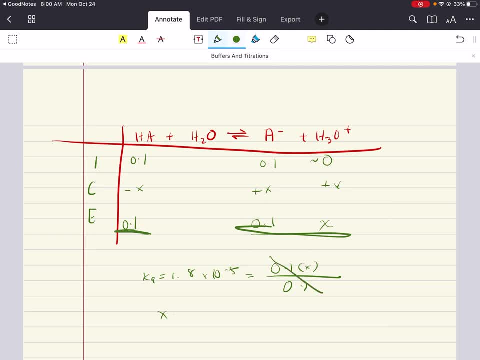 these 0.1s cancel out and x is just 1.8 times 10 to the minus five. this is our concentration of h3o, plus, by the way, because it is just x. and now, if we want to find the ph, it's just going to be. 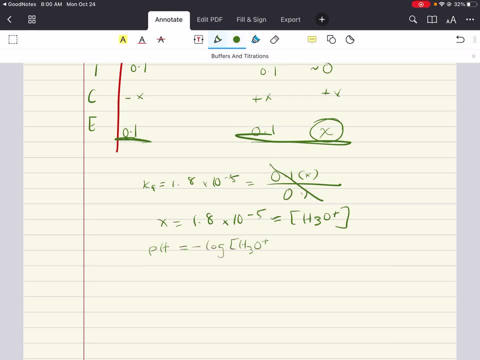 equal to the negative log of our h3o plus concentration, and that's going to get in it. so we're going to get the negative log and that's going to get in it. so that's going to get in it. so we're going to get the negative log and that's going to get in it. so we're going to get. 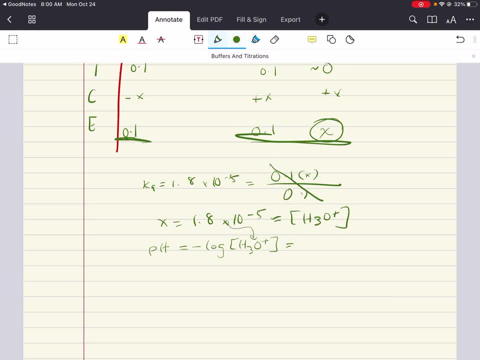 us, if we plug in this number here, a pH of 4.74.. Fantastic. Now, if 0.01 mole of HCl is added to the mixture, all right. then the H3O plus from the strong acid is going to react with the CH3COO. 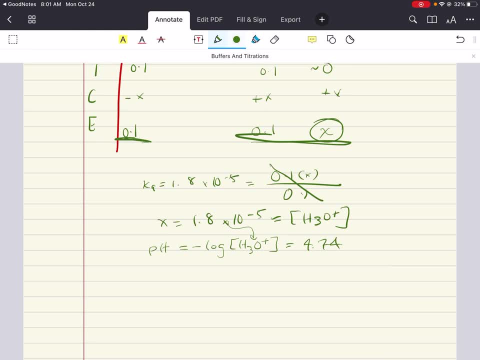 minus our acetate anion, all right. And this reaction is going to be depicted best using a one-way arrow instead of an equilibrium arrow, since the reaction between strong acid and weak base goes essentially to completion. Now we can calculate these quantities, all right. 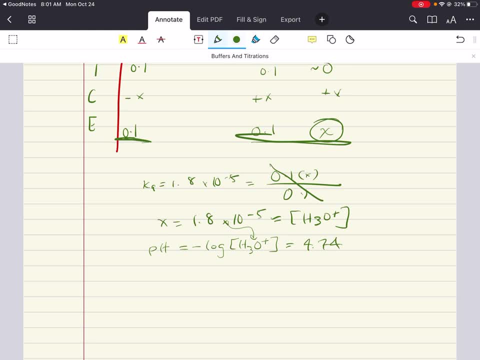 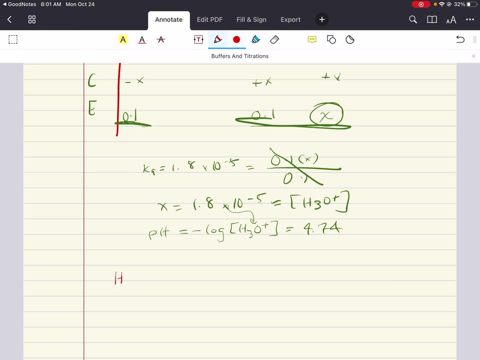 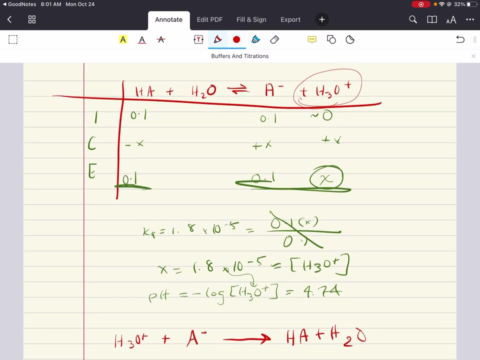 We can calculate these quantities, So by adding HCl. all right, we're going to rewrite this equation to be H3O plus plus A minus goes to HA plus H2O. all right, We're essentially doing the reverse of this. because we're adding a HCl, We're adding a. 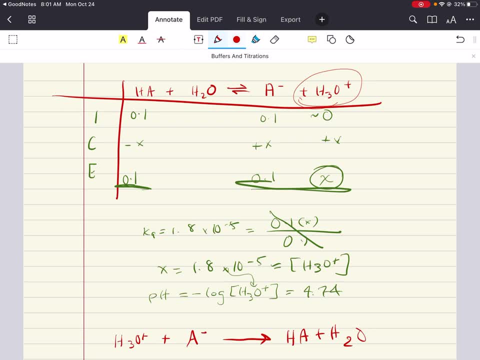 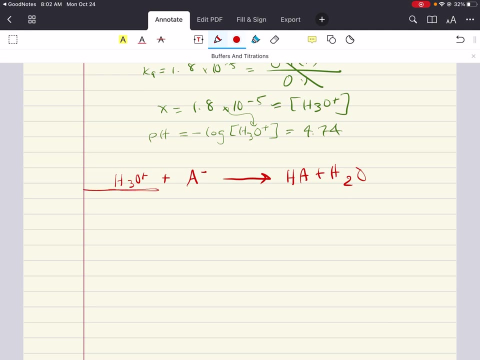 strong acid. all right. That strong acid is going to react With the anion here, the A minus. all right. So our HCl here now we're going to represent as a strong acid, which we write H3O plus. Now, the best way to solve what happens when we add. 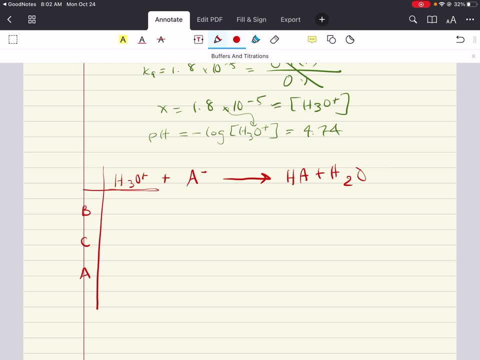 a little bit of HCl to this reaction is doing a BCA table. And now we get to introduce the BCA table. all right, It stands for before change and after, And a BCA table uses moles or millimoles. 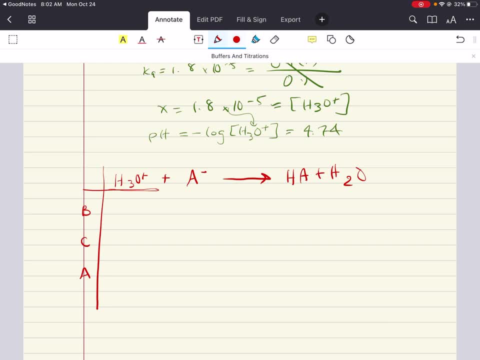 not concentrations. all right, Now it is going to be used when a reaction is best described as going to completion, like we do here. That's when we know that we can use a BCA table rather than the equilibrium ICE table. Fantastic, All right. When a reaction goes to completion. 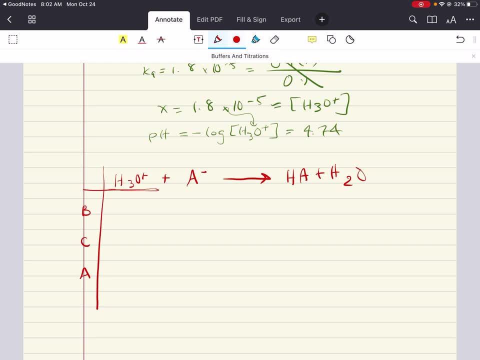 we're going to solve it using the techniques we learned for solving stoichiometry problems all the way from BCA to BCA. So we're going to use a BCA table rather than the equilibrium ICE table back in Gen Chem 1,. all right, So first we have to use moles when solving stoichiometry. 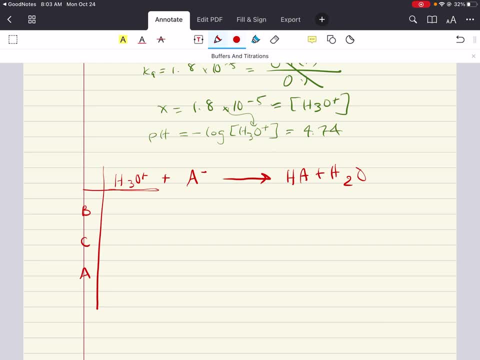 problems rather than concentrations. And second, remember that, since the reaction goes to completion, the amount of change listed on the change line is determined by the amount of limiting reactant. So in a reaction such as this, where the mole-to-mole ratio of reactants is one-to-one, 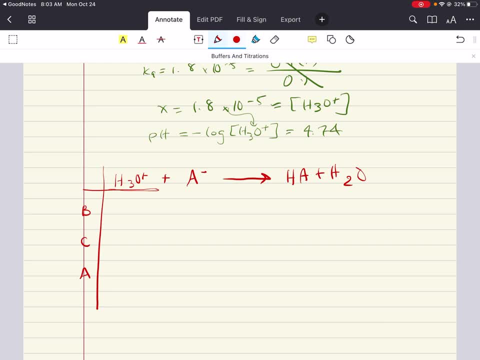 the limiting reactant is the one with the fewest number of moles, all right, So that means our limiting reactant is the HCl. is the H3O plus that we've written here? all right, Because there's fewer moles here And we're going to start by writing off all the moles. right, We're adding. 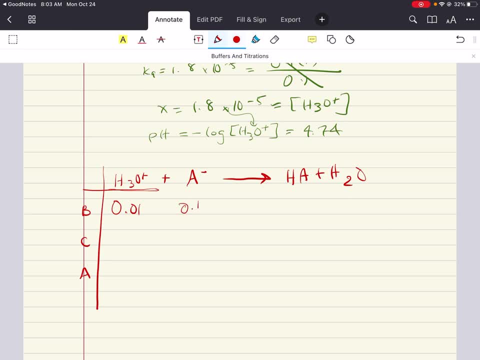 how much 0.01 mole of HCl? all right, This is 0.1, and this is 0.1.. Now, how much is 0.1?? How much is the change that's happening, like we said, all right, In this reaction? okay, since the. 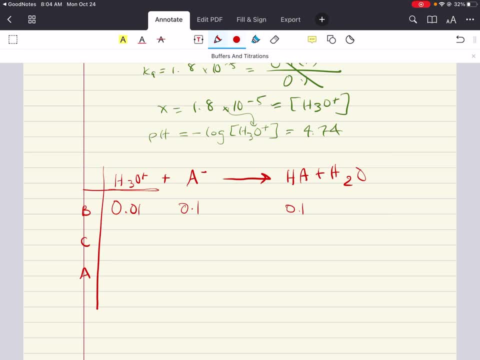 completion goes to the reaction goes to completion. the amount of change listed in the change line is determined by the limiting reactant, And here we have the fewest number of moles for the HCl. so it's going to be minus 0.01,, minus 0.01,, minus 0.01, all right. What does that give us for after? 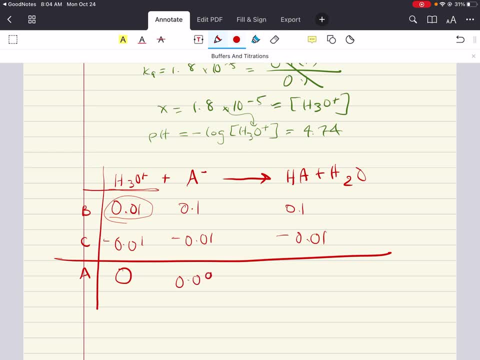 It's going to be zero. all right, This is going to be 0.09, and this is going to be. this is going to be plus. I'm so sorry. right, You lose reactants to form products, and this is going to be 0.110,. 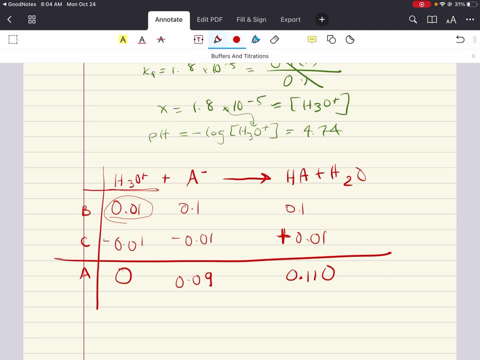 all right, Fantastic. all right. So we have all this information written here. Now we can plug the results of this stoichiometry problem into the equilibrium problem. all right? So what that means is that we have all this information written here. Now we can plug the results of this. 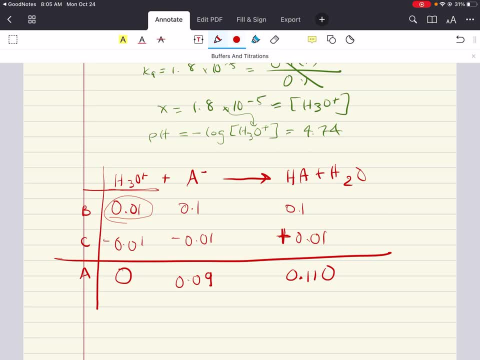 to do this, we have to convert the numbers of moles from the BCA table to concentrations for the ice table. all right, So, if you remember, we have here the volume for this. the volume of the solution for this problem is one liter, So the concentration of units that we're going to get is 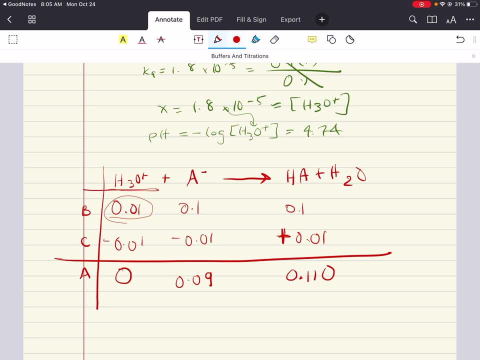 mole per liter, all right. If it wasn't one liter, you would have to determine the concentration, and that doesn't change, by the way, in this problem. If it did, or if the volumes were not one point liter, you would have to determine the concentration of the solution for this problem. 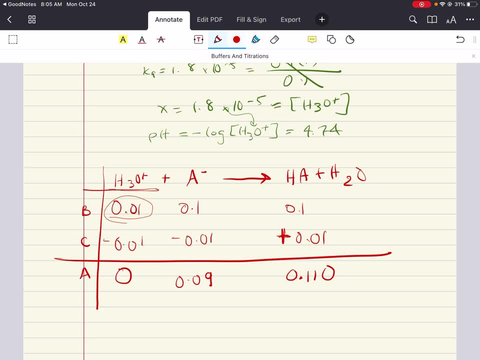 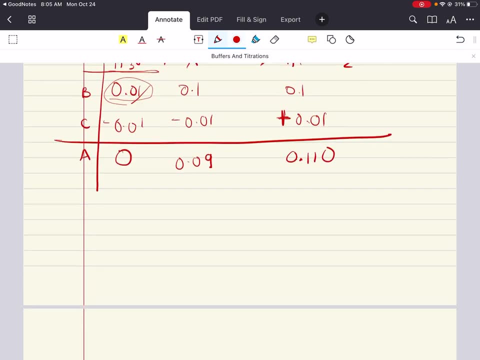 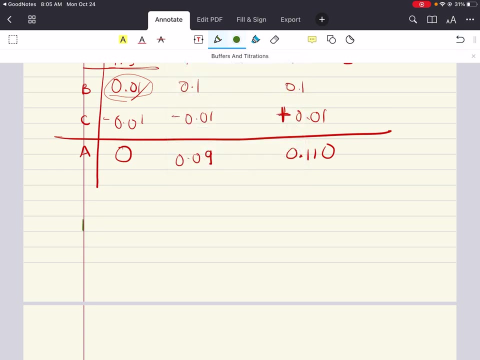 You would have to determine the concentrations of each substance by dividing the number of moles by liters. all right, So now we can take this information, plug it back into our ice table. all right, Back into an ice table, all right. I C E. Now that we've figured out. 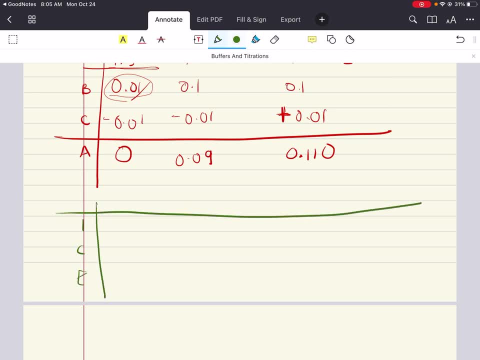 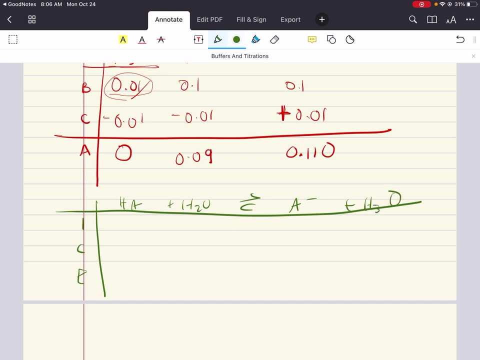 a lot of important information. okay, So HA plus H2O- equilibrium: A minus plus H3O plus H2O- all right Now when we added. well, we used our BCA table to figure out. all right Is when we added. 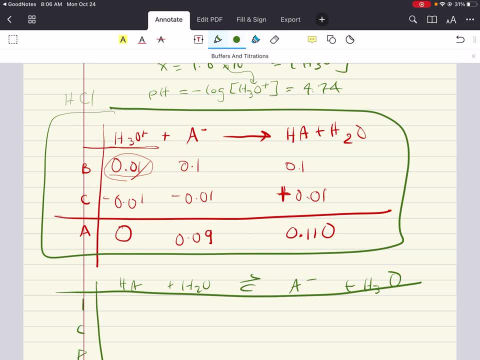 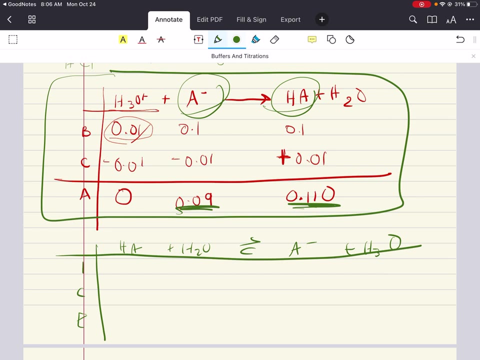 HCl. how did it change things here? How did it change this concentration? How did it change this concentration? Now we have those new concentrations and we can take them, plug them into our ice table to figure out our new pH based off of the fact that we added HCl to the mixture. 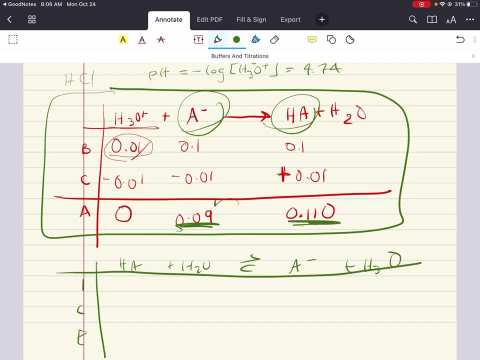 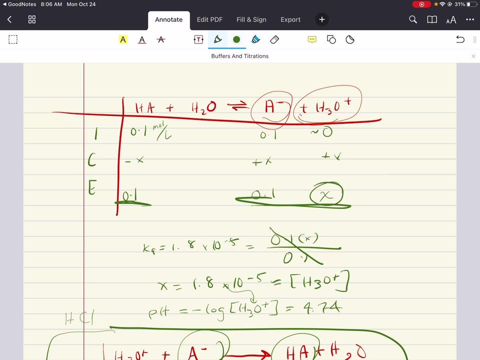 all right. Now we have our new moles here. right, Because we only work in moles in BCA tables. Now these moles were easy to write. We can still just write 0.1,. right, Because the concentration here is 0.1 moles per liter and liter is just. 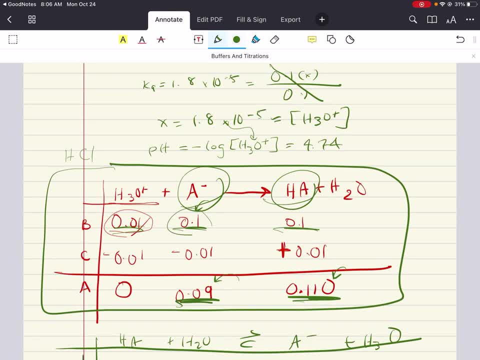 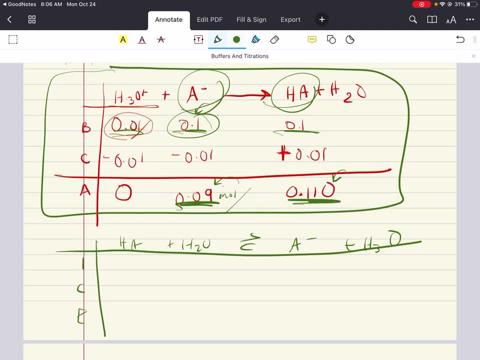 one here, So it was an easy translation. all right. Now we have to go back from these final values, which are just in moles, to molarities, to concentrations, But we only need to divide those by one liter, because this whole thing's happening in one liter, which makes the math. 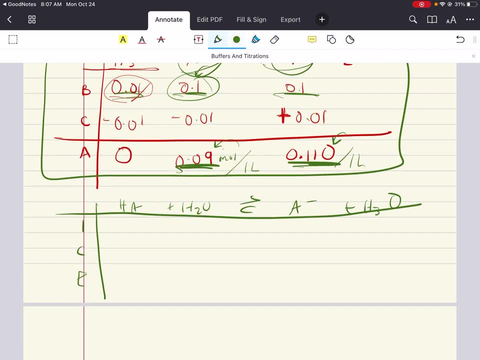 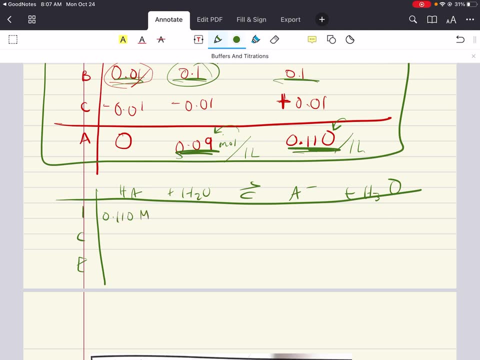 guess what? Very, very, very easy, okay. So now what we have for HA is 0.110 molar. all right, We divided that by one liter to get back our molars. Remember: this only works with moles, or millimoles You cannot use. 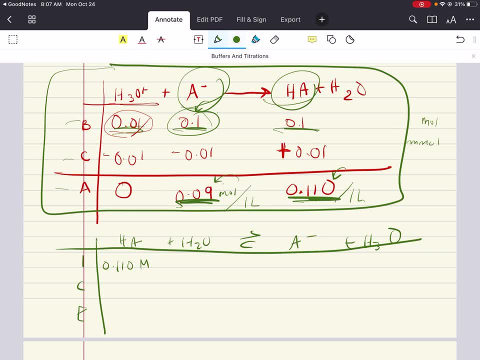 concentrations for BCA tables, all right. And then for our A minus we have 0.09 moles. We divide that by one liter and that gives us 0.09 molarity. all right, And this is approximately zero. now, 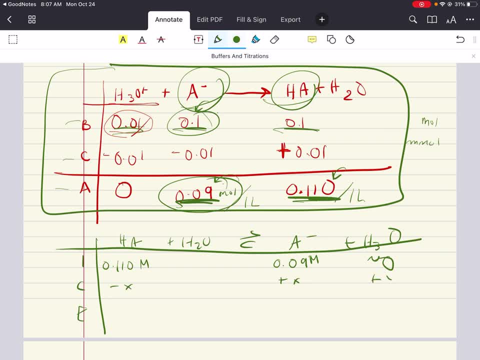 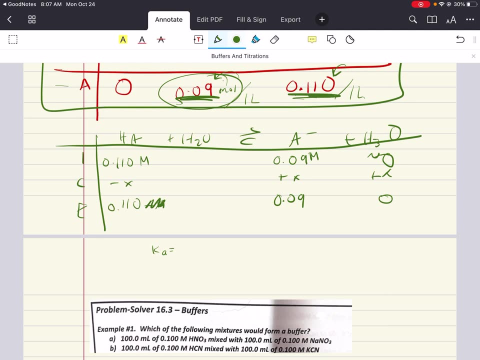 Now we lose reactants to form products and we're going to assume that X changes are negligible, so we can forget about them. all right And zero. Fantastic. Now what we can do is figure out our KA value. all right, That's. 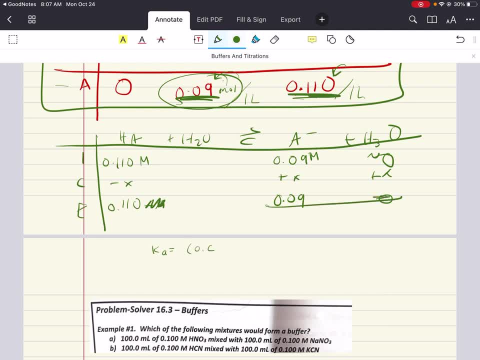 going to be products. This is plus X, I'm so sorry. Products 0.09 times X over reactants: 0.110.. This gives us a K value of 1.8 times 10, to the minus 5, because that's our KA value. Now we need to solve for X. X is equal to 2.2. 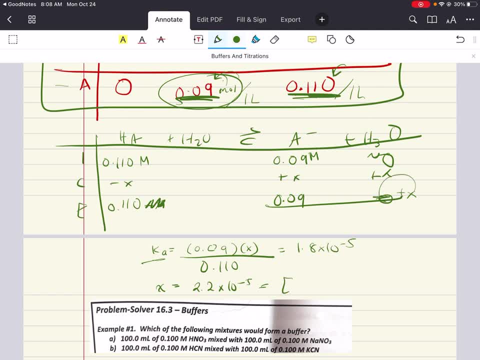 times 10 to the minus 5, which is, by the way, because H3O plus is plus X. this is our H3O plus concentration. And now we can find the pH by doing the negative log of the H3O plus. 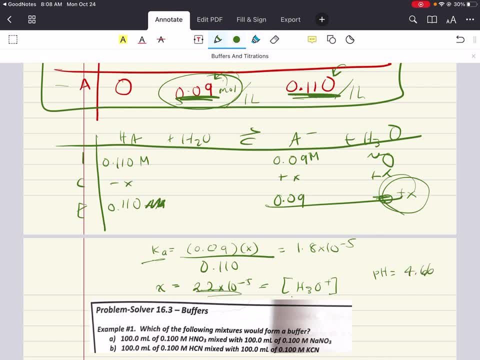 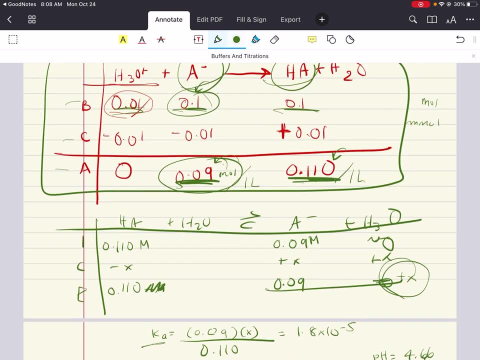 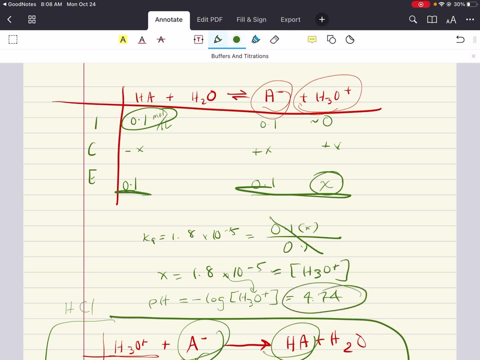 concentration and that gives us a pH of 4.66.. Compare the results of those two problems, guys. When we were just doing, when we were just doing all right without adding H3O, it was 4.74,. all right, Adding H3O. 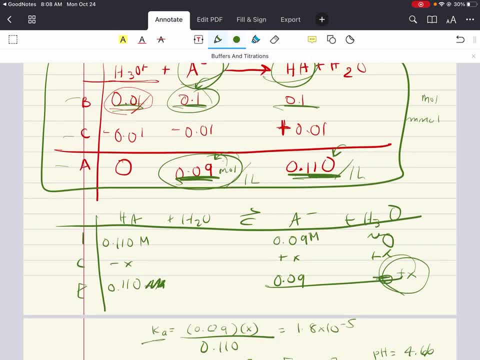 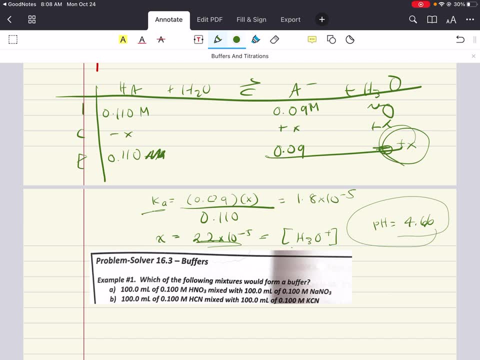 our pH barely changed. all right, 4.66,. only a difference of 0.08 pH units. Compare this to when we added H3O to just pure water. Our pH went from 7 to 2,. all right, It jumped 5 pH units. In the other hand, here: 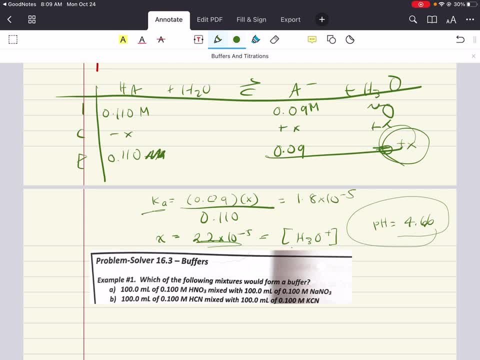 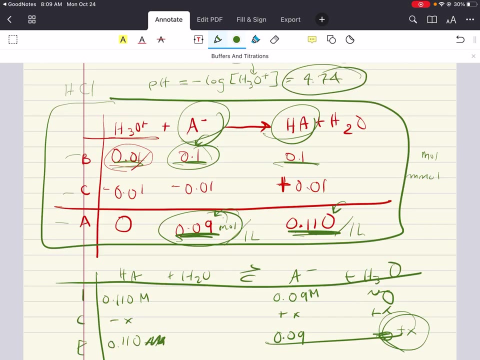 our pH only jumped 0.08 pH units. all right, Because our buffer solution worked pretty well at mitigating the effects of adding any acid or base to that solution. all right, So that's how buffers work. all right. Now I'm going to scroll back up here. There's a few. 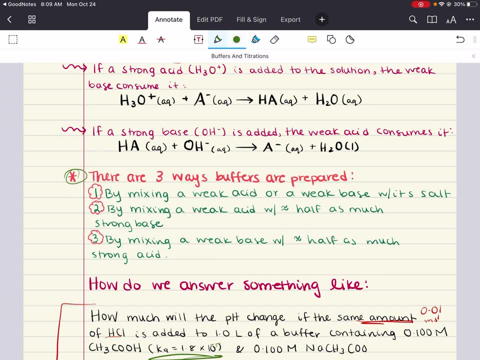 important notes. we skipped To do this problem, and that's how buffers are prepared. okay, A buffer exists anytime a weak acid and its conjugate base are present in the solution in roughly equal amounts, like we saw in this problem. all right, There are three ways that a buffer can be prepared. 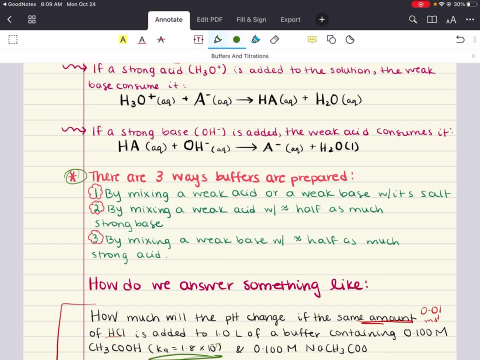 Buffers can be prepared: one by mixing a weak acid with its salt- all right. or a weak base with its salt- all right. That's one way. Two buffers can be formed by mixing a weak acid with approximately half as much strong. 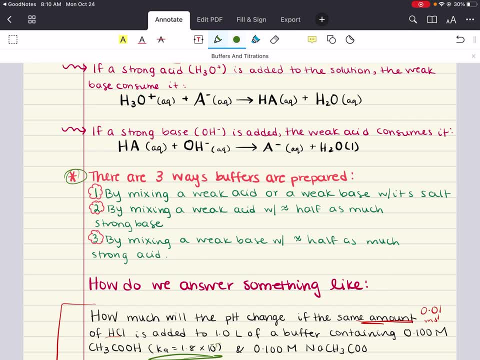 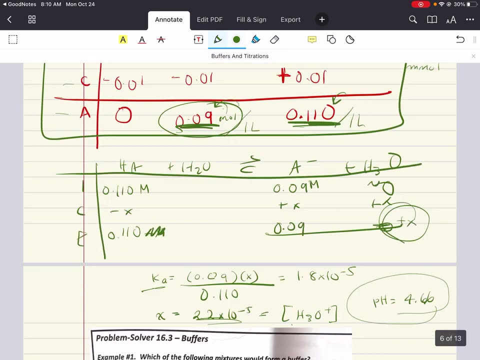 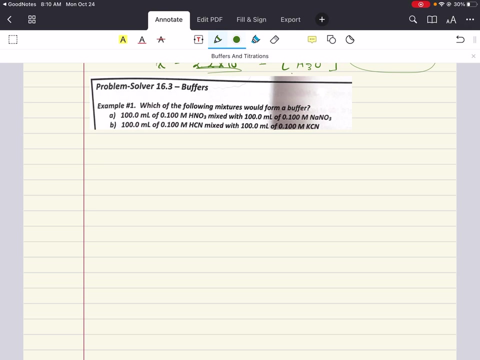 base, all right. And third, we can form a buffer. if a weak base is mixed with approximately half as much strong acid, all right, The resulting solution is going to form a buffer. Fantastic, Fantastic. Now let's do a buffer problem. all right, Which of the following mixtures would form a buffer? So, 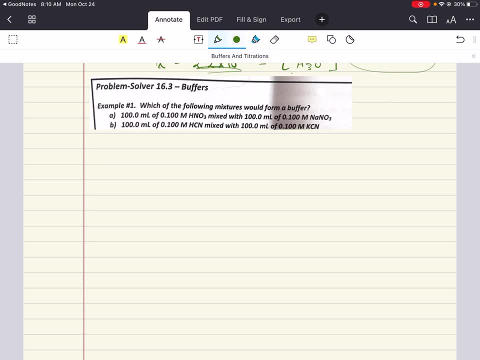 let's do A: 100 milliliters of 0.1 molar HNO3 mixed with 100 milliliters of 0.1 molar NaNO3,. all right. Any solution containing a weak acid and its weak conjugate base will act as a buffer. 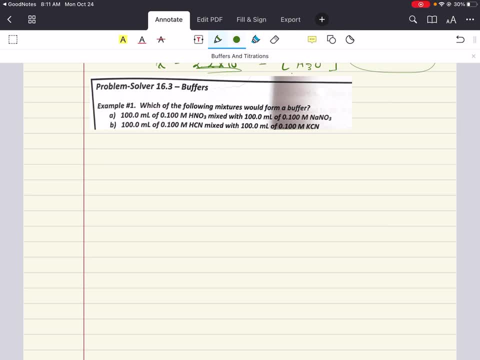 Therefore, to determine if this mixture will form a buffer, we need to consider the species present in solution. all right, Remember HNO3, if you remember from your list that you had to memorize of strong acids, this is one of them. all right, This is a strong acid. When a strong acid. 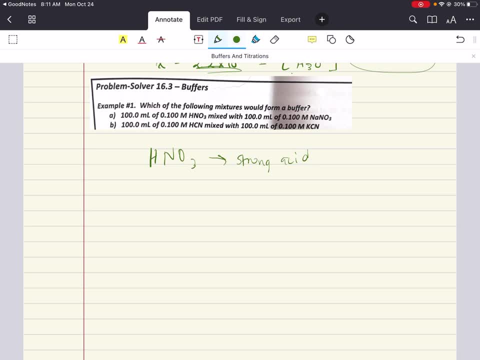 ionizes in aqueous solution, it completely dissociates. So when HNO in water completely dissociates, all right, we're going to form NO3- plus H3O+. Now Na, sodium nitrite, NaNO3, sorry, this is a soluble salt And in solution. 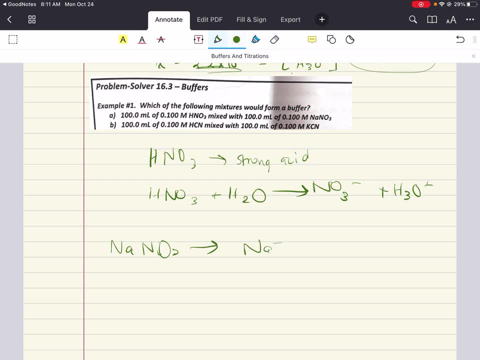 it's going to dissociate. It's going to dissociate into Na+ plus NO3-. all right, The sodium here is a spectator ion. Therefore, when HNO3, nitric acid is mixed with sodium nitrate, the following species are going: